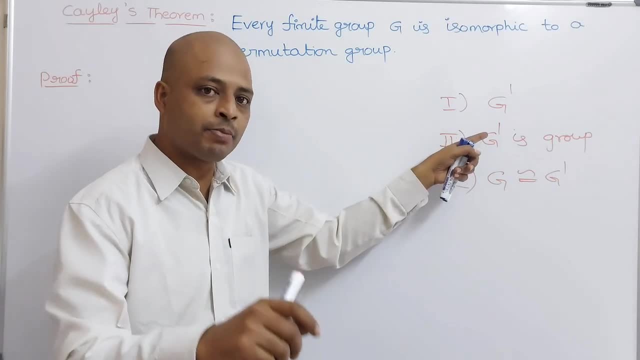 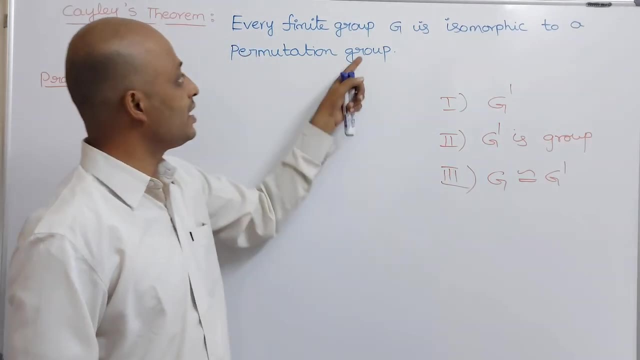 we prove that this set G' is a group under permutation multiplication. In the step 3, we prove that this G' is isomorphic to G'. That is, finite group G is isomorphic to the permutation group G'. 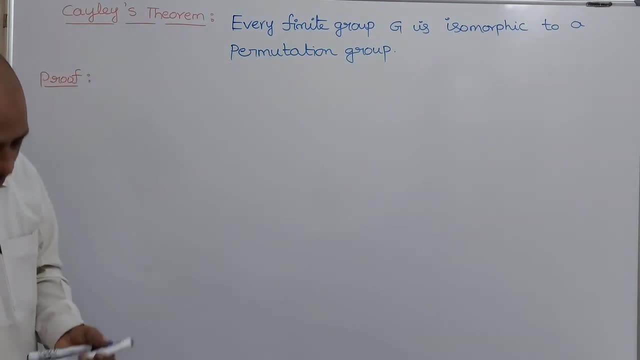 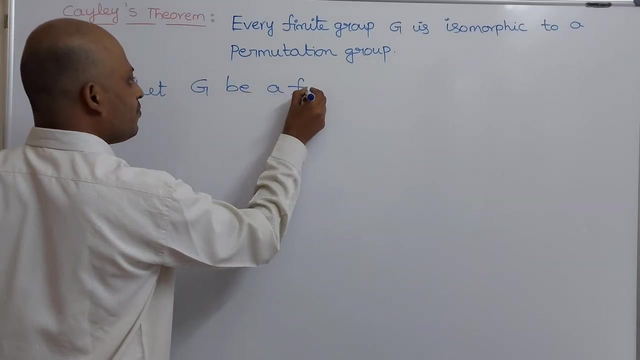 Let us start our proof. Let capital G be a finite group. Let capital G be a finite group. 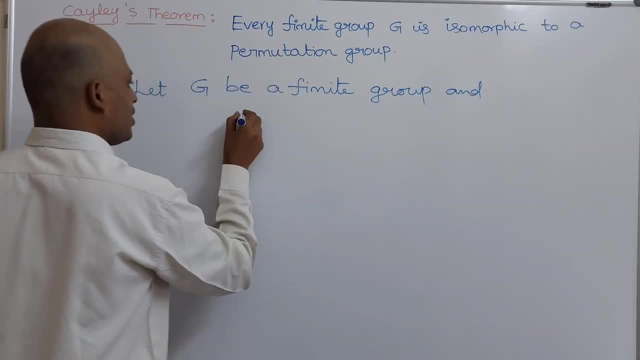 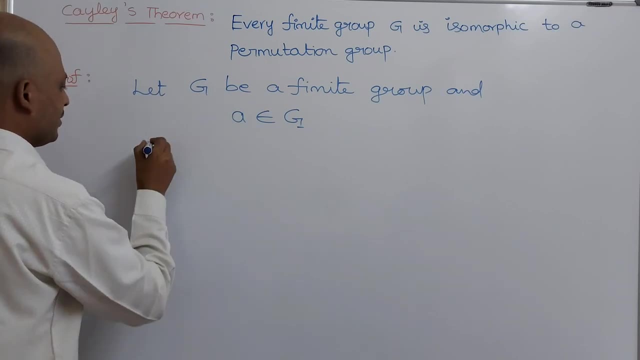 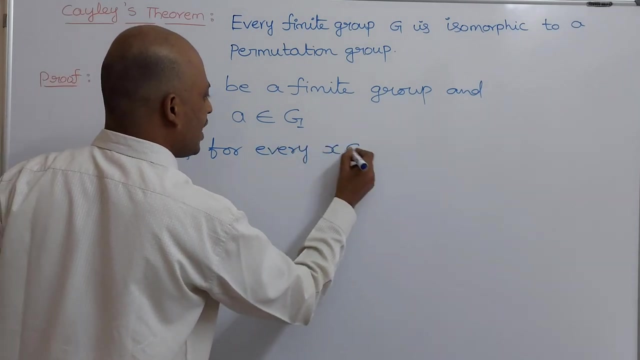 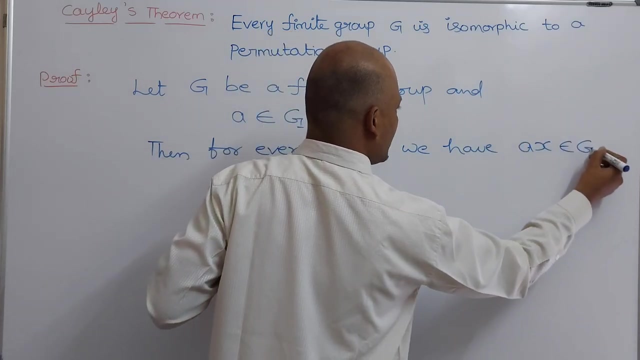 And small a belongs to capital G means small a is an element of G. Then, for every x belongs to capital G, we have For every x belongs to G, we have a x belongs to capital G. 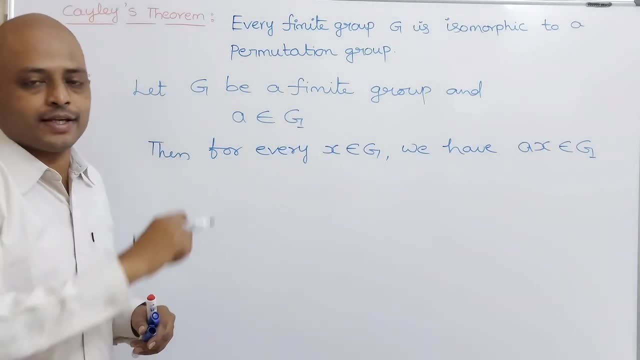 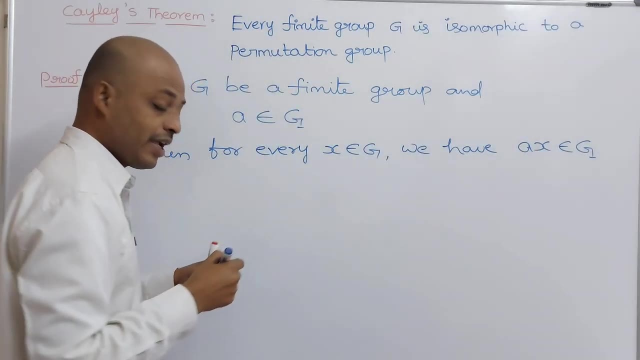 Because G is a group, by applying closure axiom, by applying closure axiom under multiplication, a x belongs to capital G for every x in capital G. 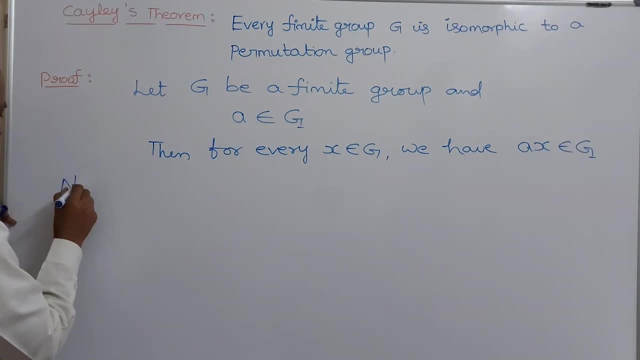 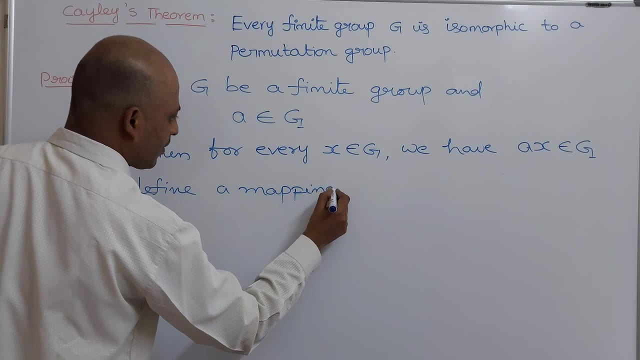 Now, define a mapping. Now, let us define a mapping. Let us define a mapping F that maps from G into G. 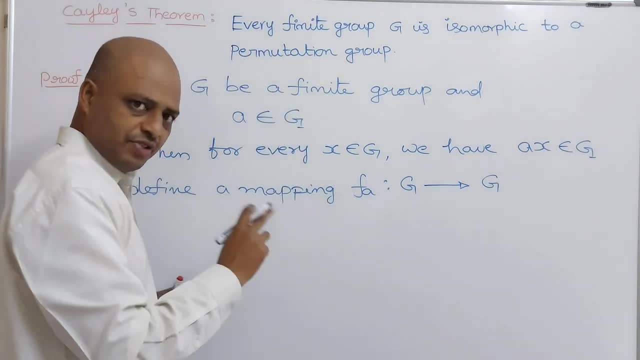 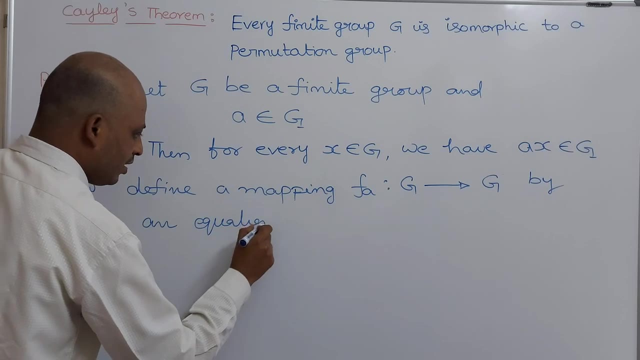 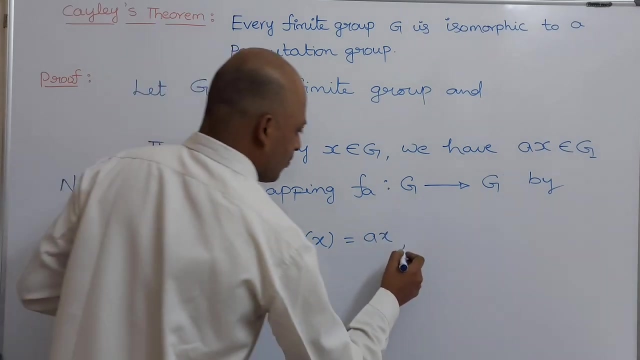 Let us define a mapping F that maps from G into G. By an equation f of x is equal to ax. 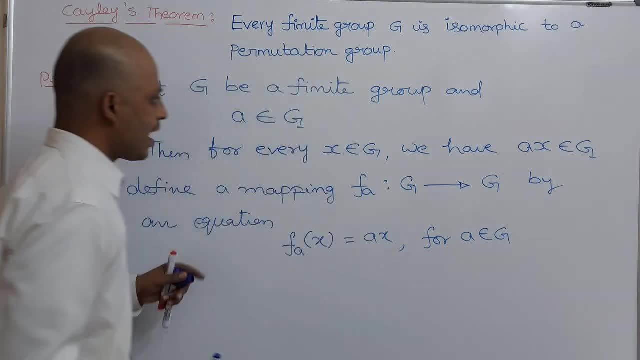 For small a belongs to capital G. For small a belongs to capital G. 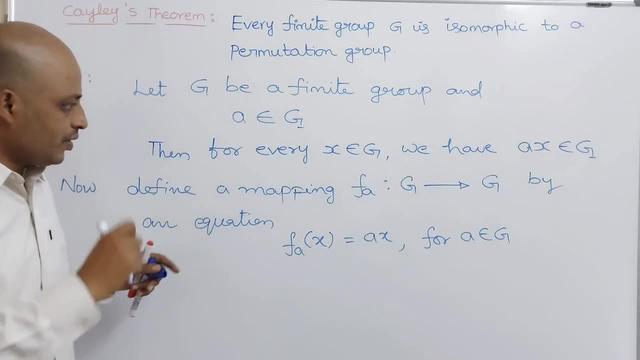 Observe that corresponding to the element A belongs to capital G, we define a mapping F of x that maps from G into G. 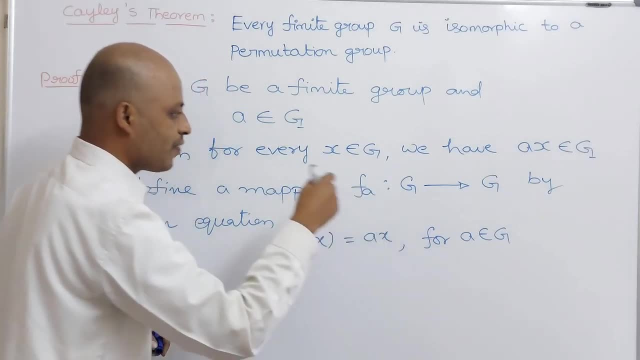 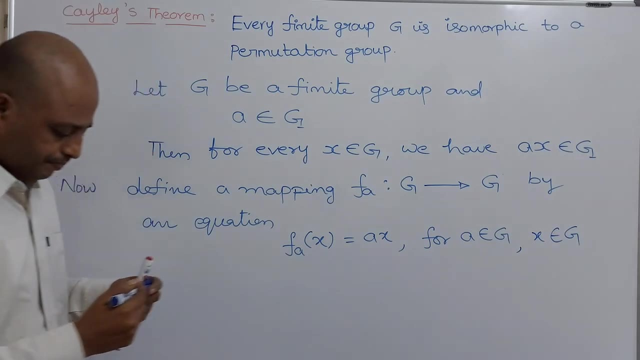 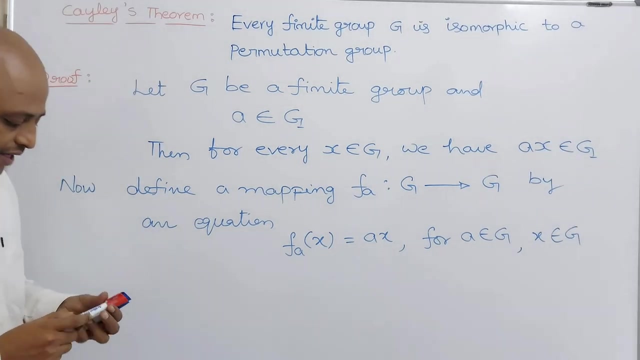 such by an equation F A of x is equals to A x for A belongs to capital G and x also belongs to capital G. Now, we show that this mapping F A is well defined. First, we show 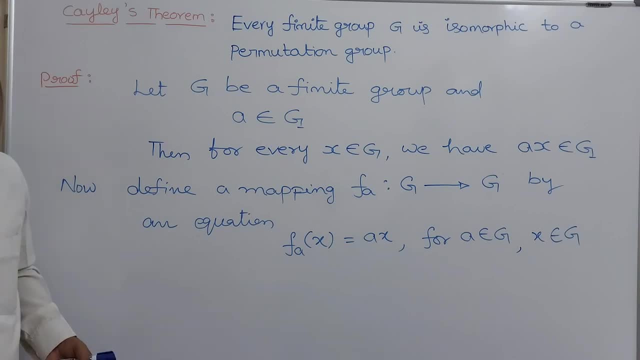 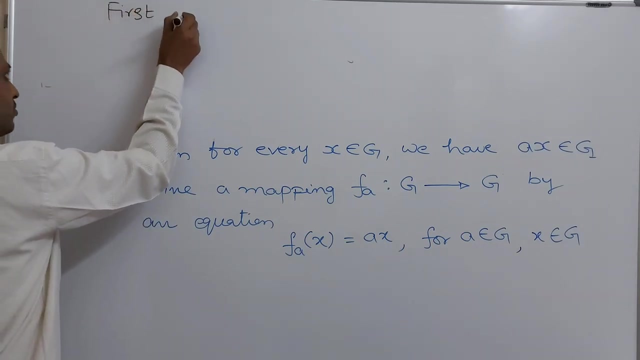 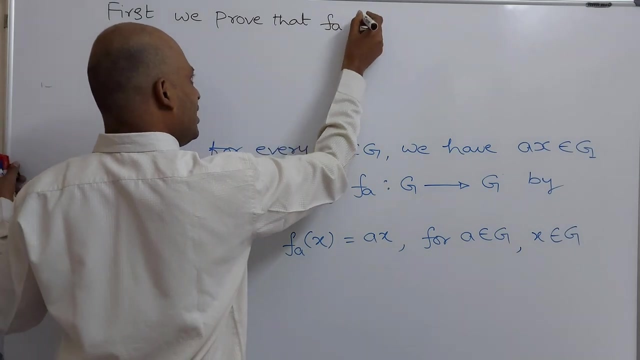 that this mapping F A is well defined. First, we prove that the mapping F A is well defined. The mapping F A is well defined. 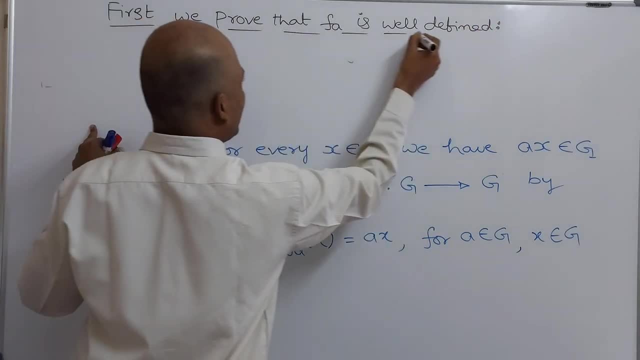 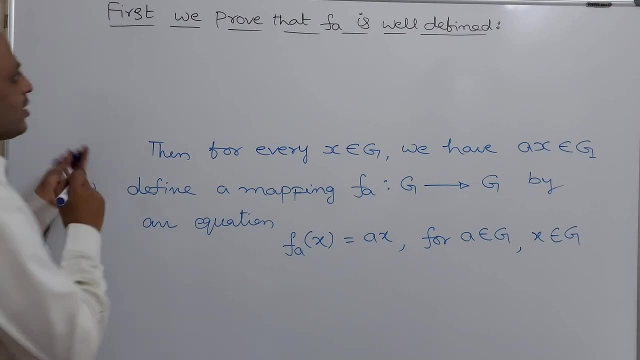 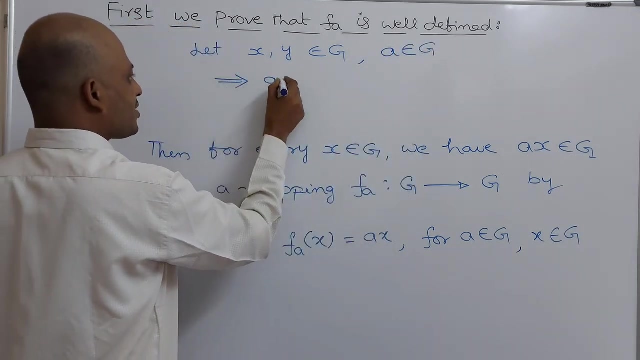 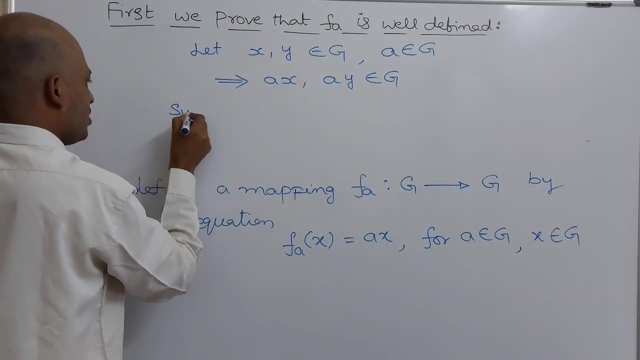 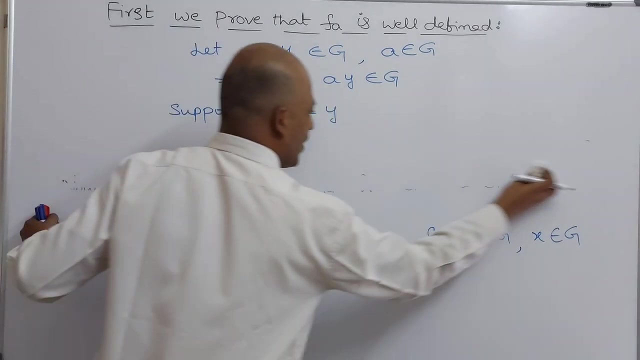 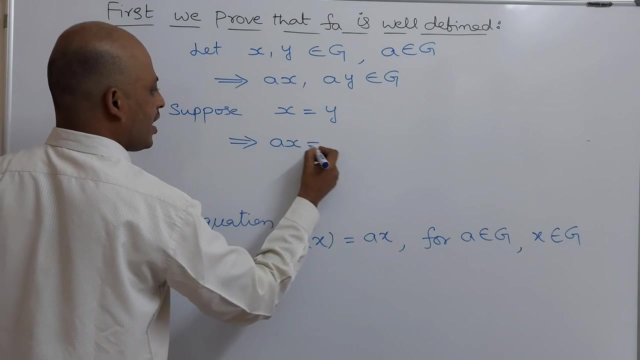 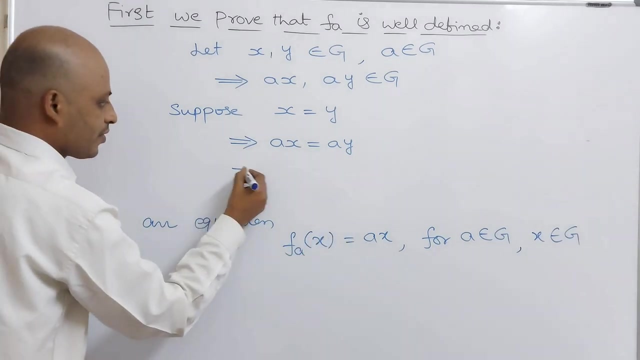 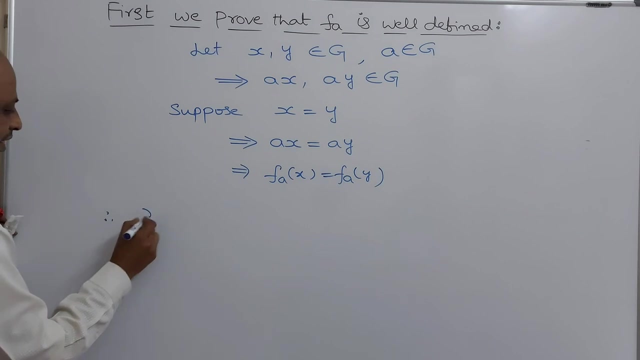 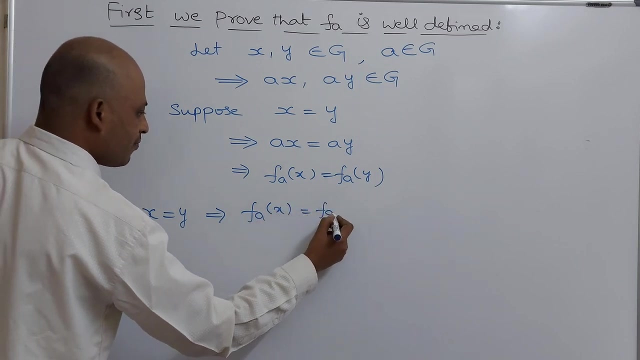 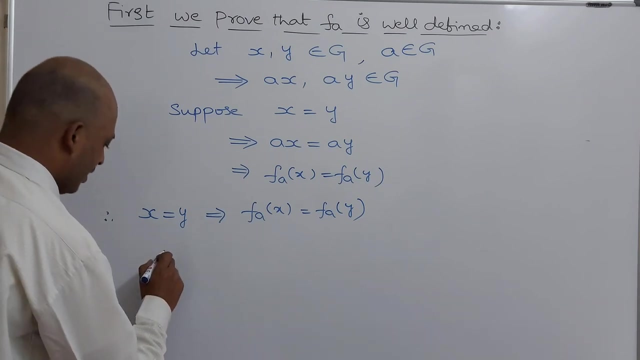 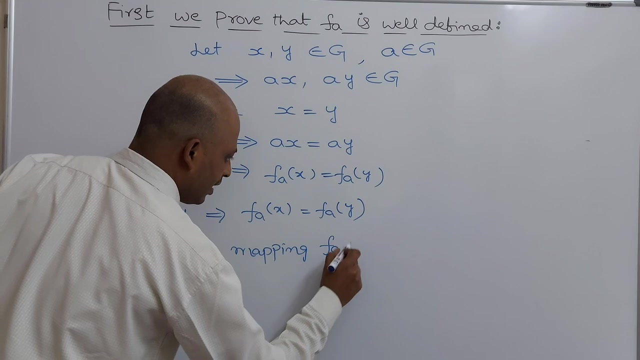 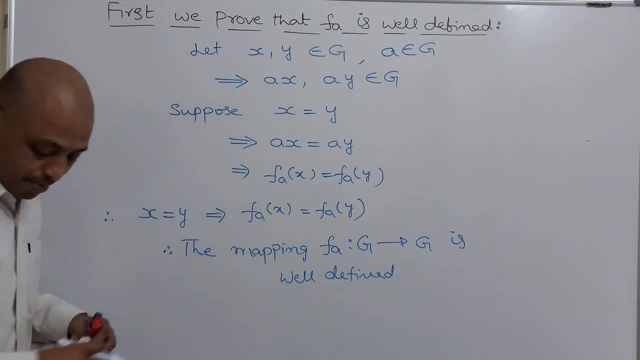 Is well-defined. Yes. The mapping which is defined like this F A, F maps A to A, F A 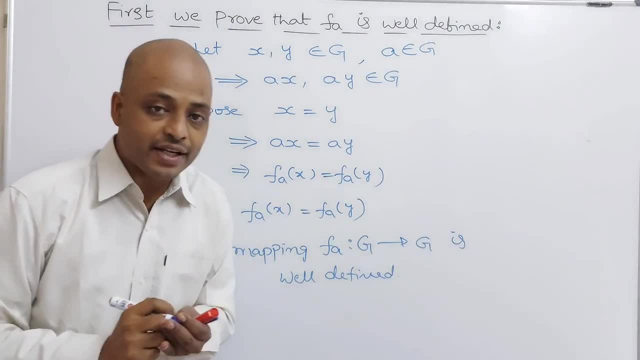 of x is equals to A x is clearly a well-defined mapping. 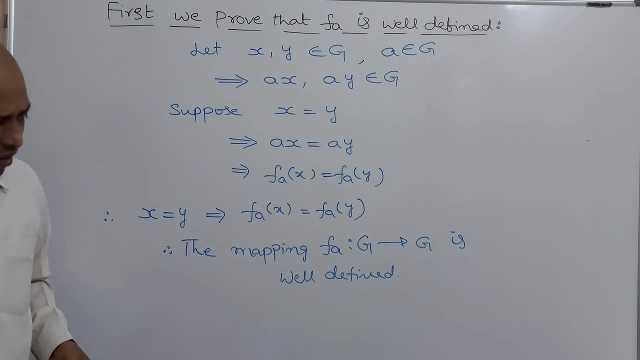 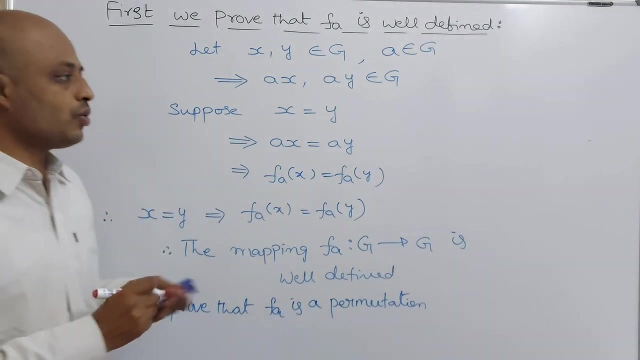 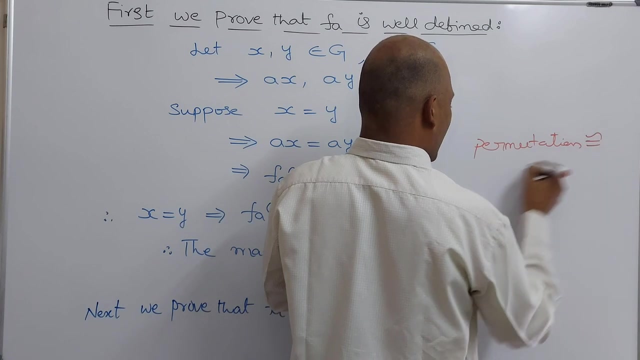 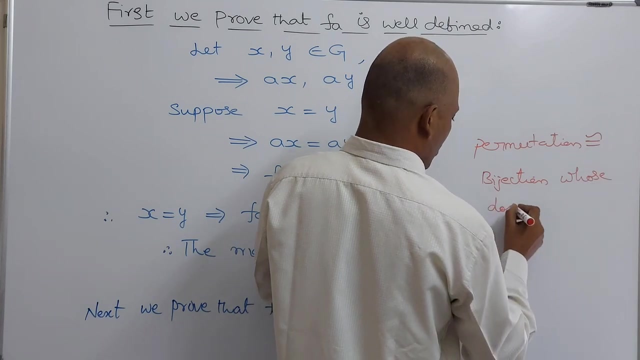 Next, we prove that this mapping F A is a permutation. Next, we prove that F A is a permutation. F A is a permutation. What is the definition of permutation? Permutation is nothing but a mapping which is both 1, 1 and 1, 2. Permutation is nothing but a mapping from a set into itself, which is both 1, 1 and 1, 2. Permutation, permutation, it is nothing but a bijection, a bijection whose domain and co-domain is same. Whose domain and co-domain is same. 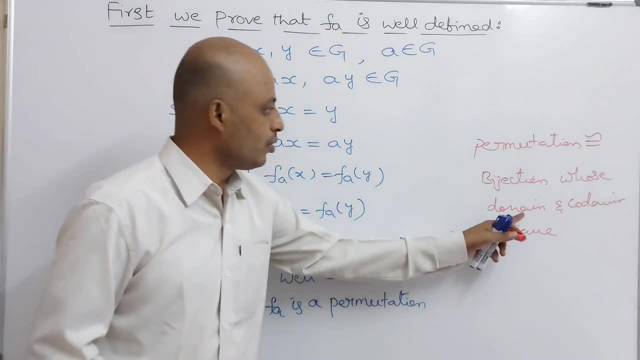 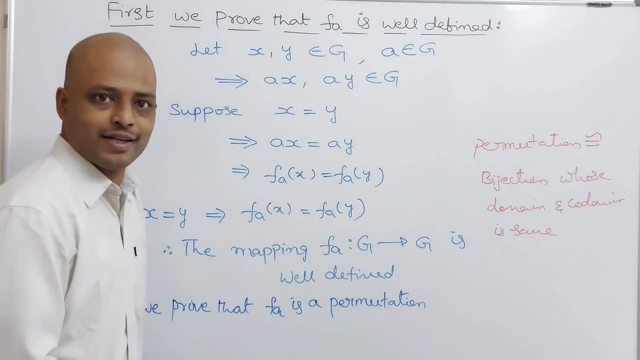 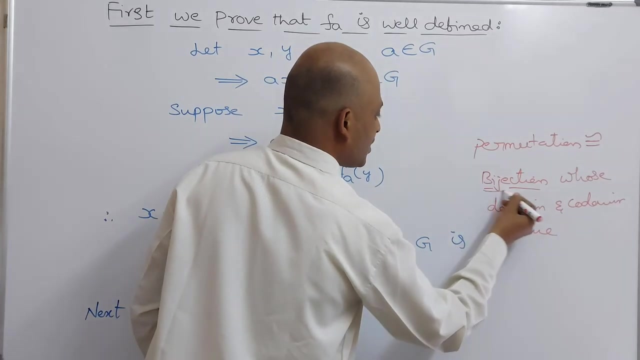 You observe that F A, F A maps from G to G, the domain and co-domain is same. We have to show that F A is a permutation. It means you have to prove that it is a bijection. 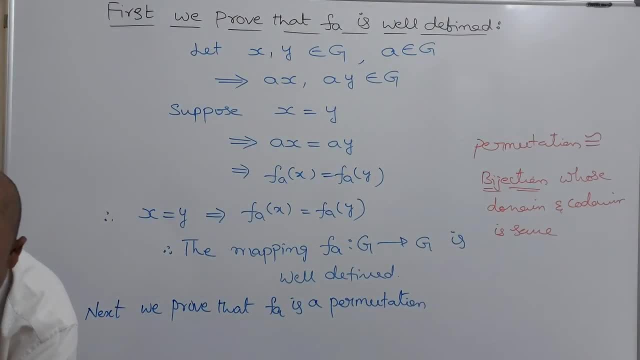 It is a bijection. Again, what is mean by bijection? What is mean by bijection? Bijection is nothing but both 1, 1 and 1, 2. 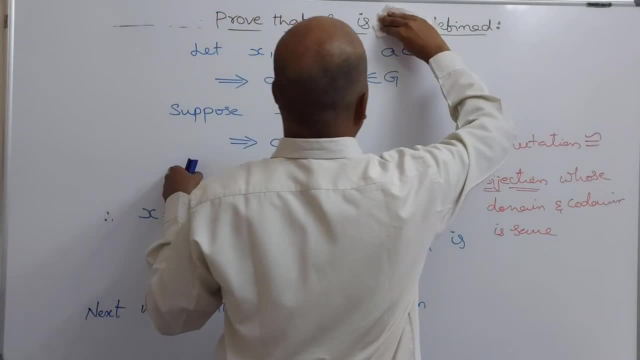 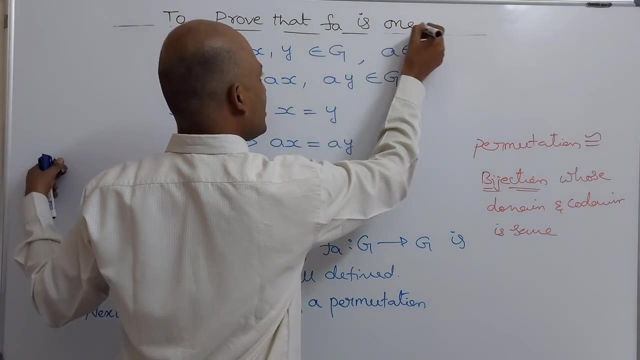 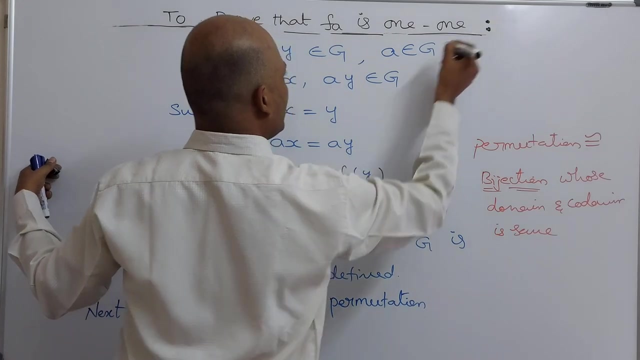 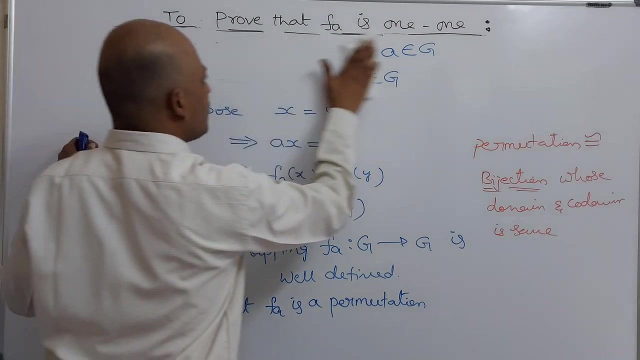 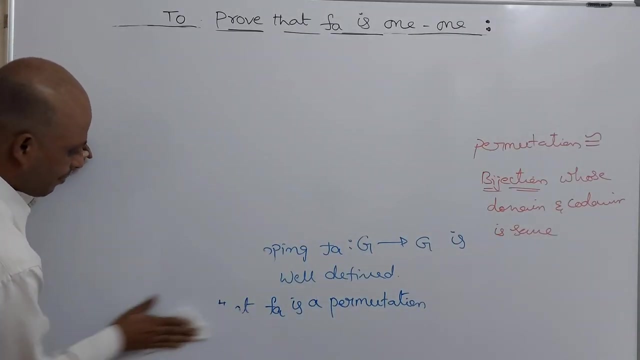 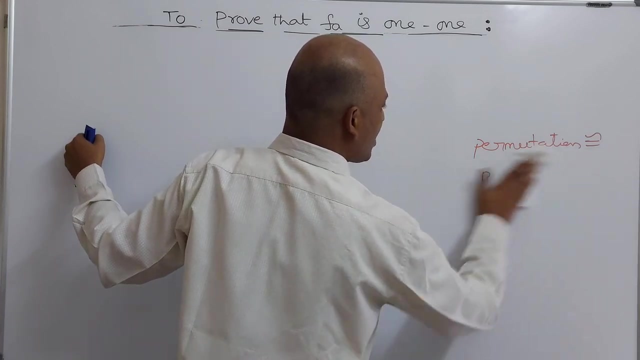 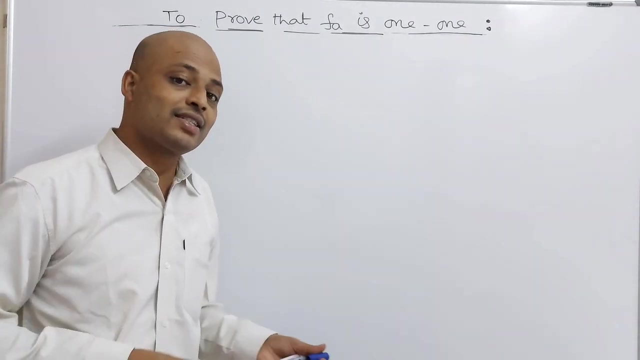 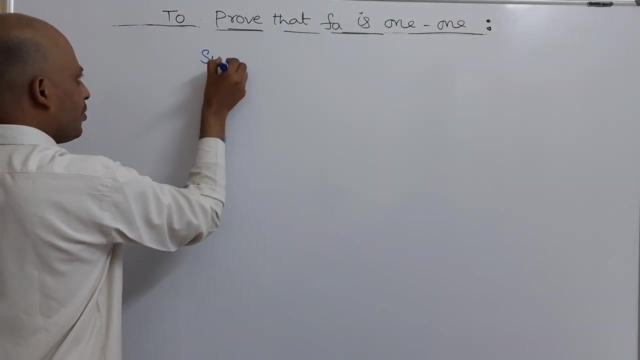 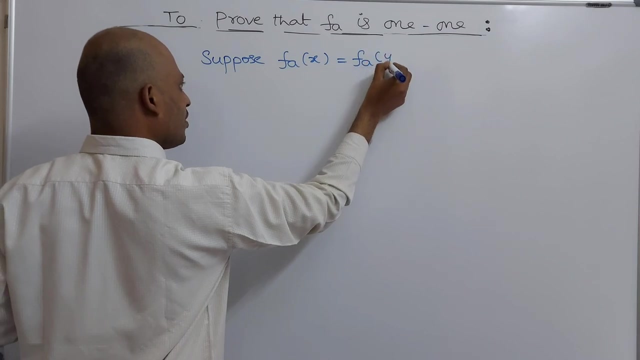 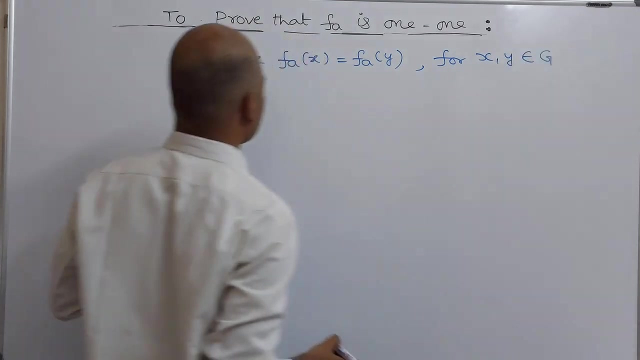 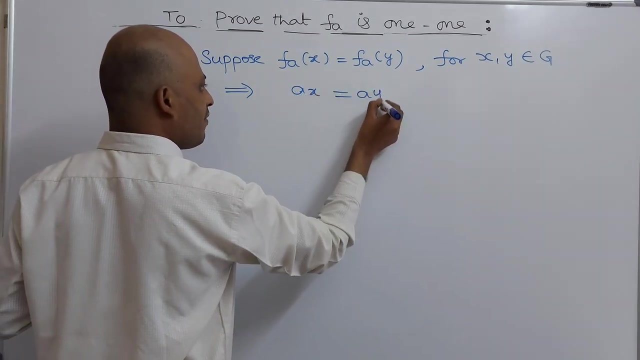 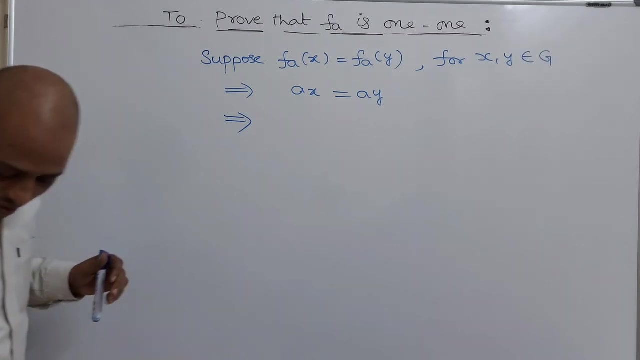 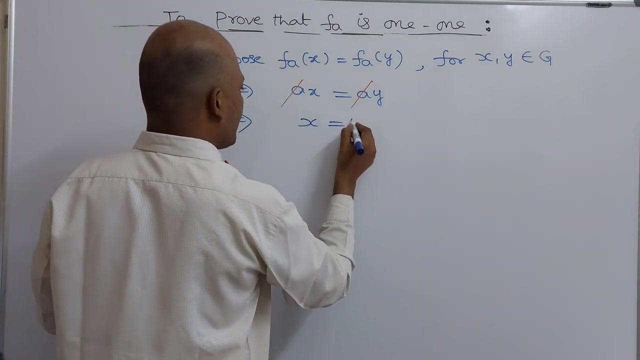 To prove that F A is a permutation, we have to prove that F A is a bijection. To prove that F A is 1, 1. To prove that, to prove that F A is 1, 1. Write your notes by using side headings, then it is very clear and easy. So write, to prove that F A is 1, 1. What is the definition of 1, 1? A mapping is said to be 1, 1 mapping. A mapping is said to be 1, 1 mapping. 1, 1 mapping. If the distinct elements of the domain has distinct images in the co-domain. A mapping is said to be 1, 1. If distinct elements of the domain has distinct images in the co-domain, then it is said to be 1, 1. So write, suppose, suppose F A of X is equals to F A of Y. Suppose F A of X is equals to F A of Y. For x, y belongs to G. By definition of the mapping, F A of X is nothing but AX. F A of Y is nothing but AY. Because G is a group, applying the left cancellation law. By applying the left cancellation law, you get X is equals to Y. Therefore, F A of X is equal to F A of Y. 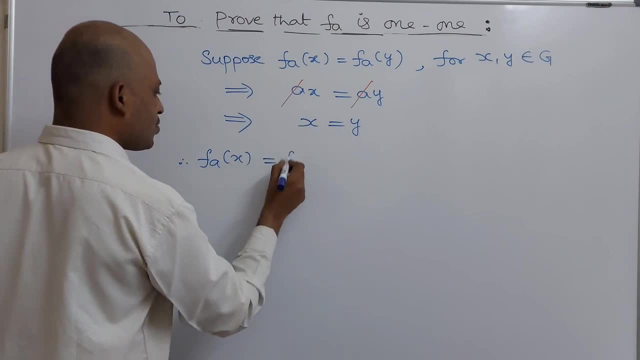 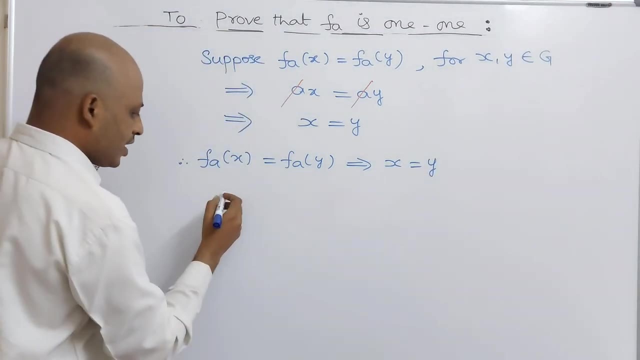 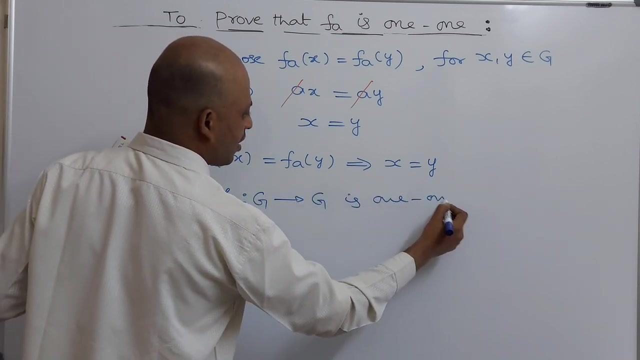 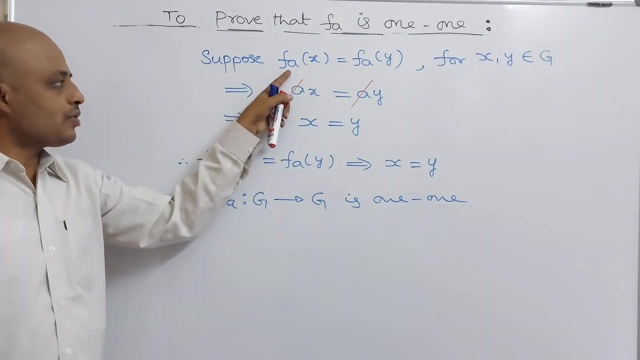 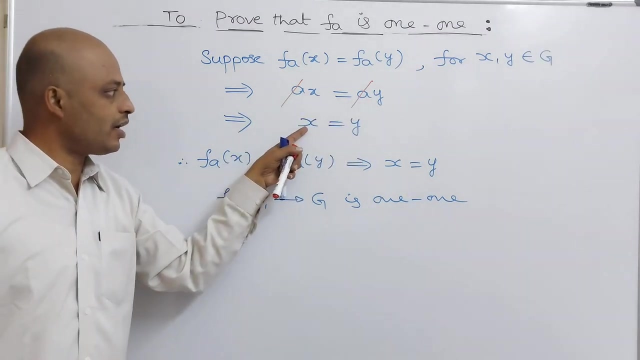 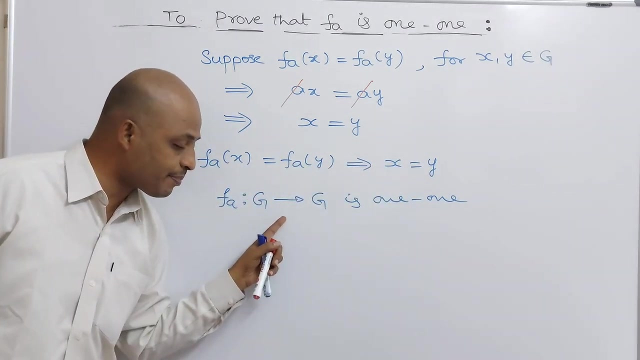 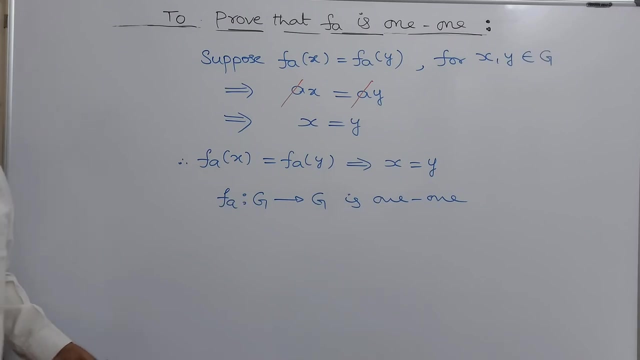 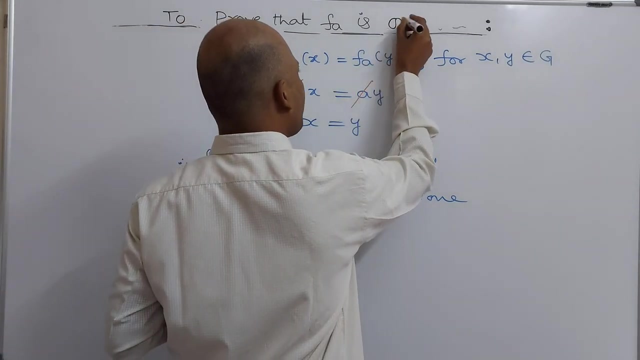 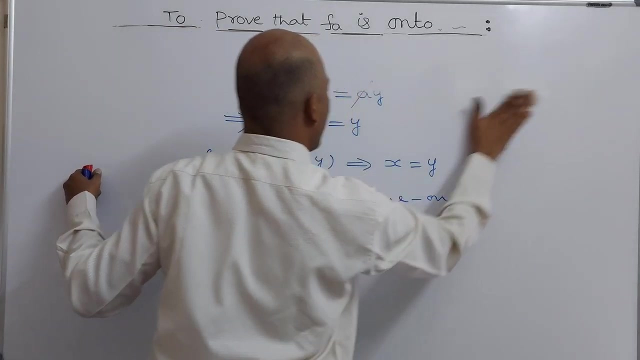 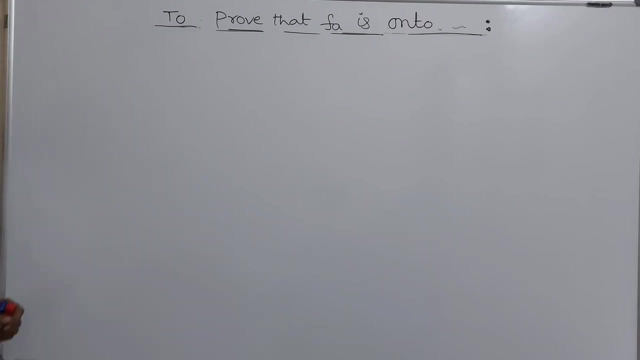 Therefore, F A of X is equal to F A of X. Therefore, F A of X is equal to F A of Y. So, same, say, F A of X is equal to F A of Y implies as X is equals to Y. состояниL This condition shows as the mapping F A Maps G to G is 1, 1. The mapping F A Maps G to G is 1, 1. So, to prove that F A is 1, 1, suppose if F A of X is equals to F A of Y, to a y. Apply the left cancellation law. You get x is equals to y. So, f a of x is equals to f a of y implies x is equals to y. This shows us the mapping f a is 1 1. This shows us the mapping f a is 1 1. Next, we prove that the mapping f a is onto. Next, we prove that the mapping f a is onto. What is the definition of onto? A function is said to be onto function. If every element of the codomine has at least one preimage in the domain. What is the definition of onto? Every element of the codomine has at least one preimage in the domain. So, right? Let us take an element x belongs to capital G codomine. Let us take an element x belongs to capital G codomine. 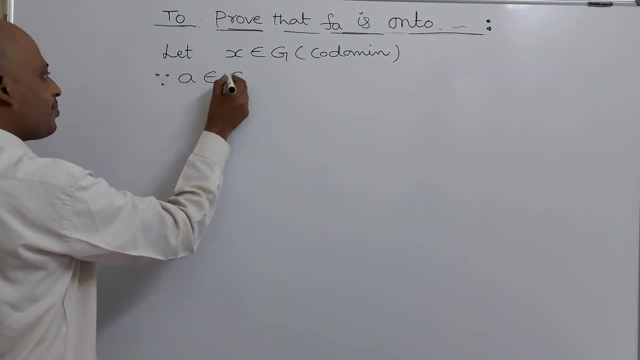 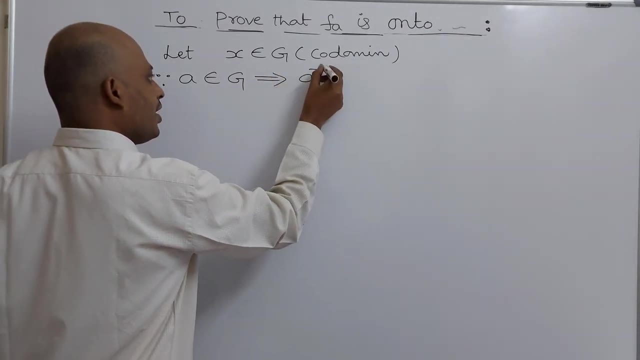 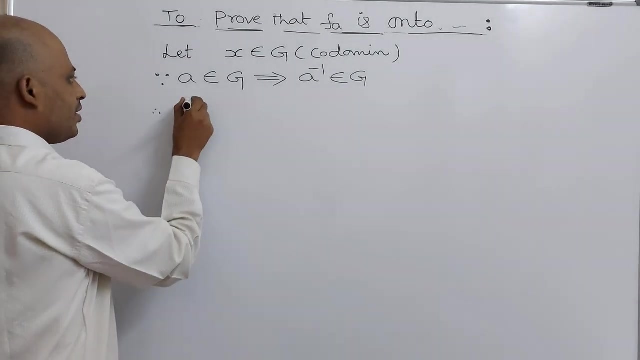 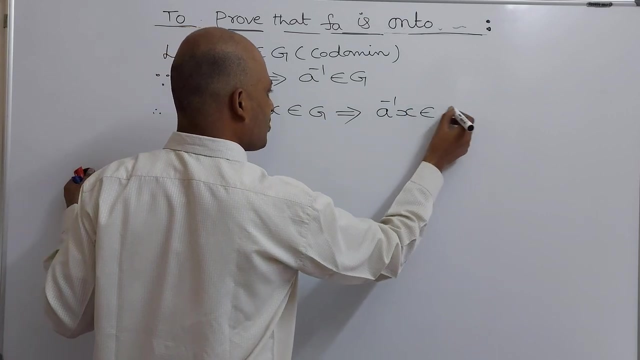 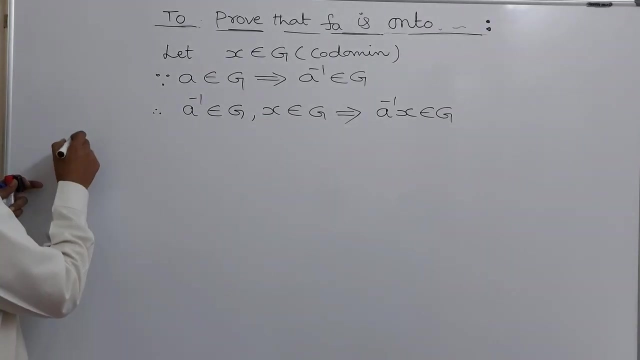 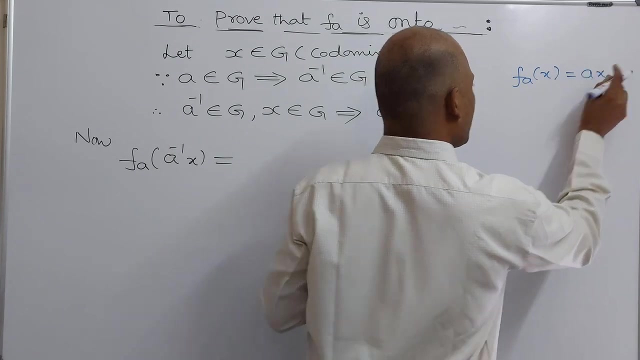 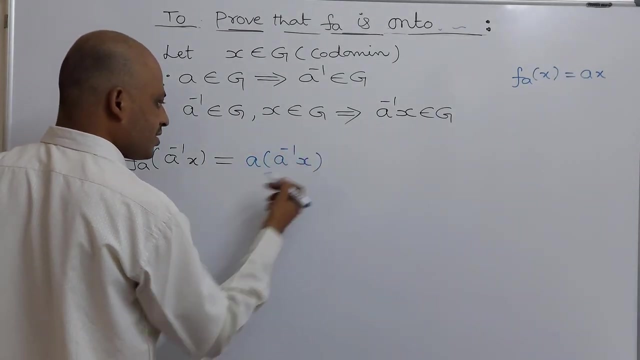 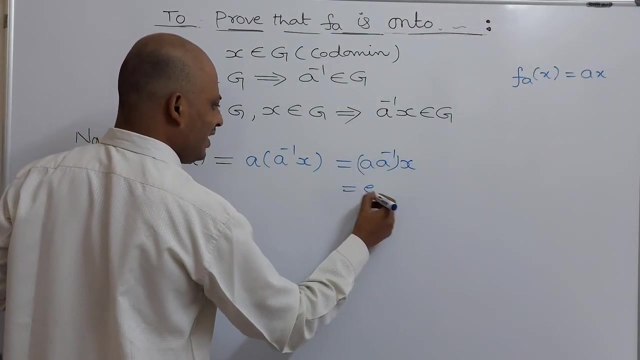 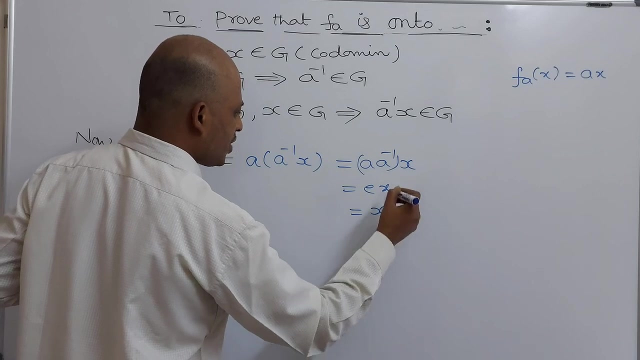 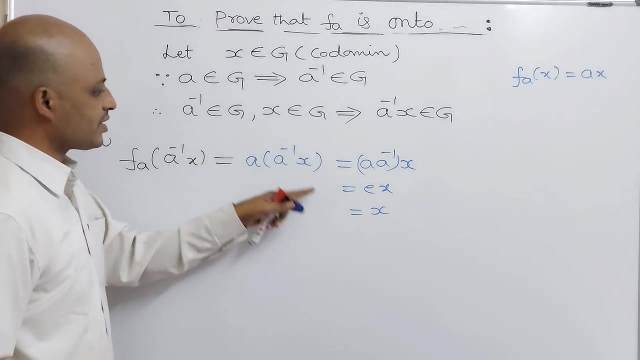 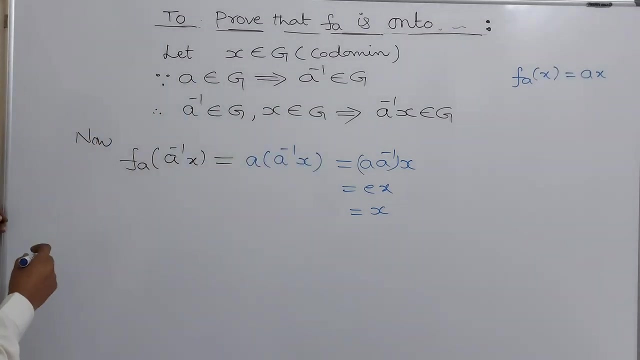 Right? Since small a belongs to capital G. And G is a group. Apply the inverse axiom. Apply the inverse axiom. a power minus 1 belongs to capital G. Now, you observe that. Now, you observe that. A inverse belongs to capital G. X also belongs to capital G. G is a group. Apply the closure axiom. Apply the closure axiom to these two elements. You get a inverse belongs to capital G. A inverse x belongs to capital G. A inverse x belongs to capital G. This a inverse x belongs to capital G. Now, calculate the value of f a of a inverse x. f a of a inverse x. What is the definition of f a? f a of x is equals to a x. By applying this definition here, f a of a inverse x is equals to a into a inverse x. Apply the associative axiom. a into a inverse x. e x. Where e is identity element in the group G. Where small e is identity element in the group G. You get x. f a of a inverse x is equals to a into a inverse x. It is equals to x. It is equals to x. You observe that now. You observe that now. 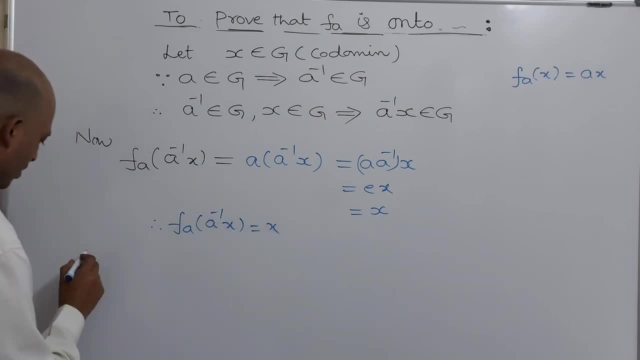 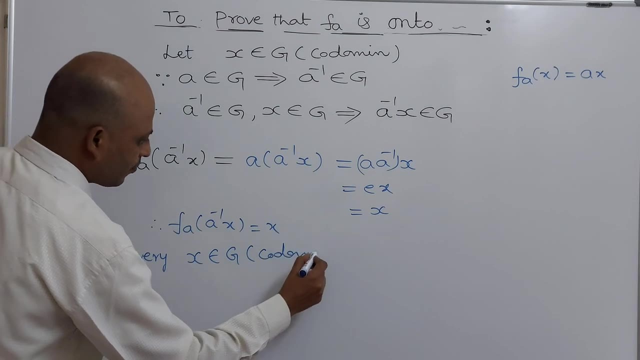 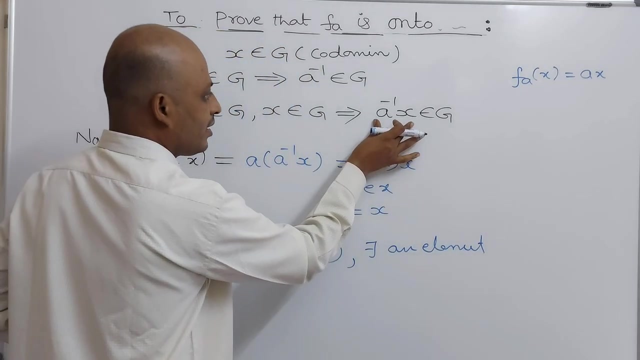 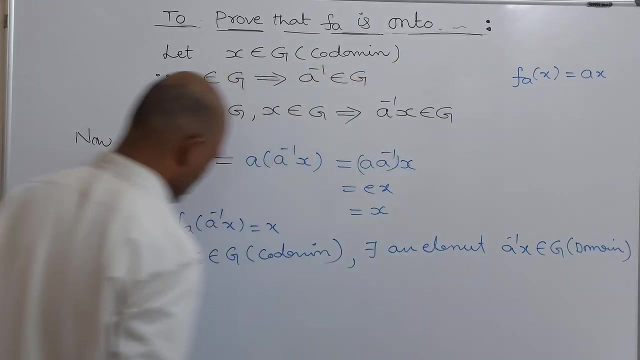 Therefore, f a of a inverse x is equals to x. For every x belongs to capital G, co-domine, there exists an element. A inverse x belongs to capital G, domain, domain, such that it satisfies the condition. f A of a inverse a x belongs to capital G, domain, domain, domain. By applying this definition, Š is the boundary. 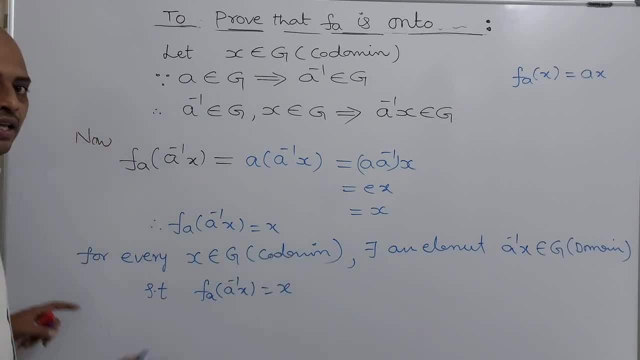 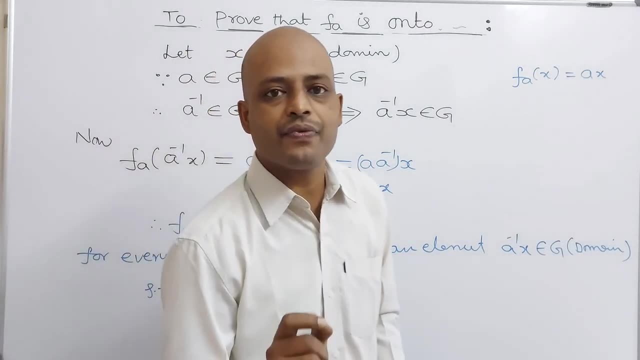 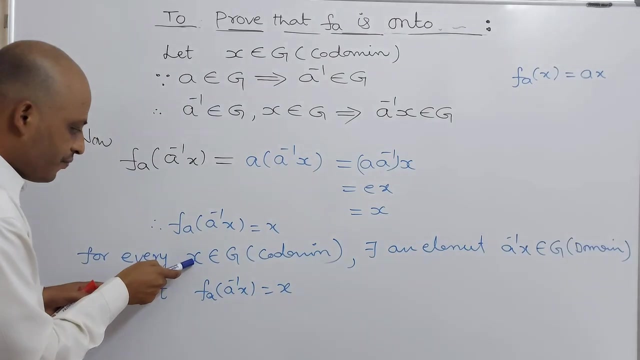 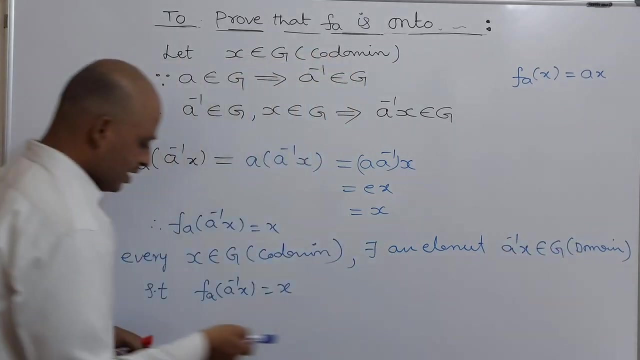 For every x belongs to capital G, co-domine, domain, domain, there exists an element. A x is equals to x. This is nothing but the definition of onto. Onto function means a function is said to be onto function if every element of the co-domain has at least one pre-image in the domain. Every element of the co-domain, every element of the co-domain x belongs to capital G has at least one pre-image a inverse x belongs to G in the domain such that fa of a inverse x is equals to x. This shows us, this shows us fa is onto, fa is 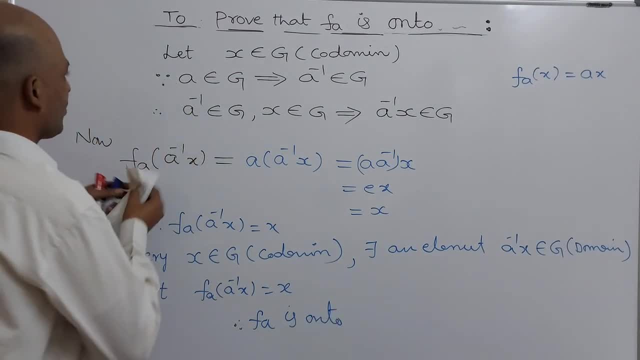 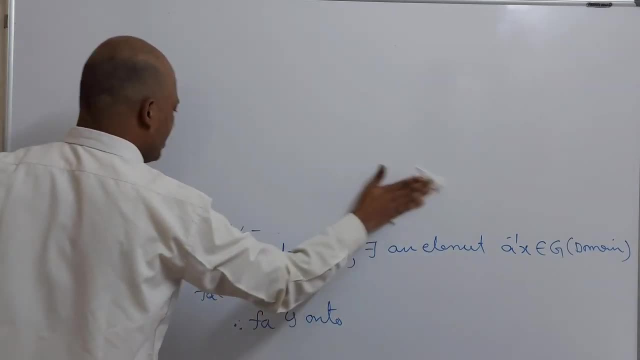 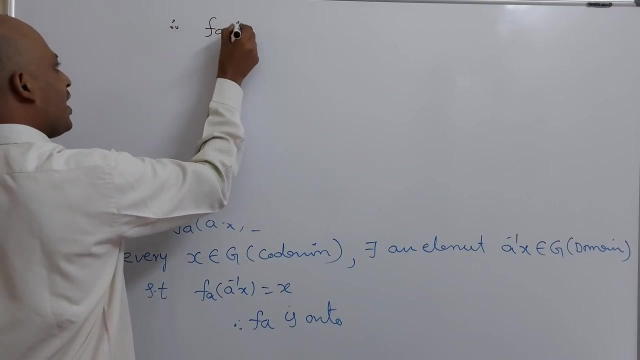 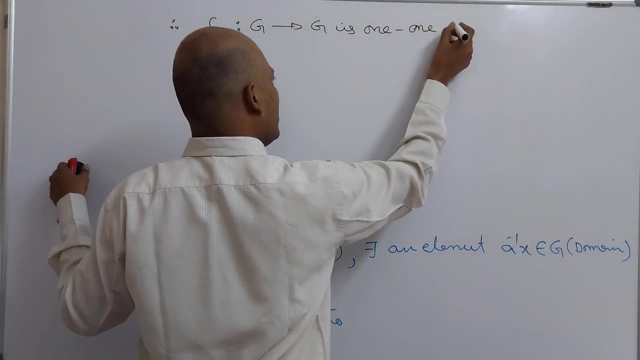 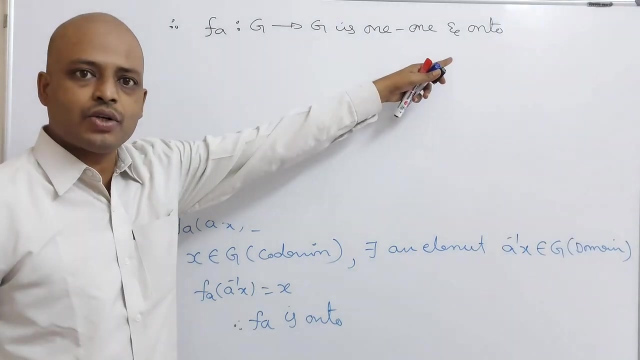 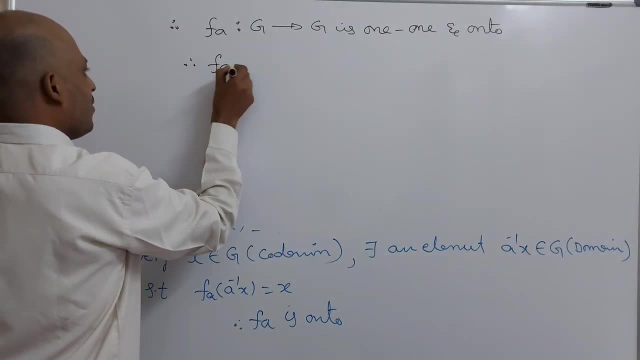 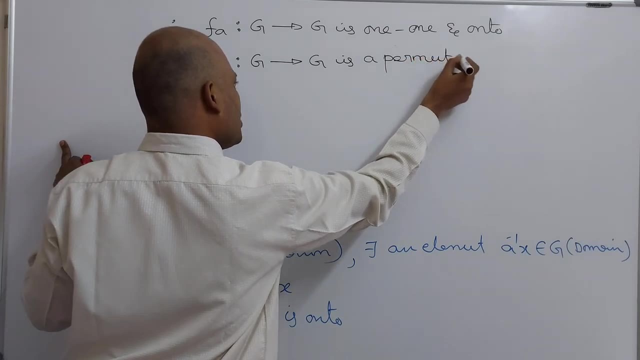 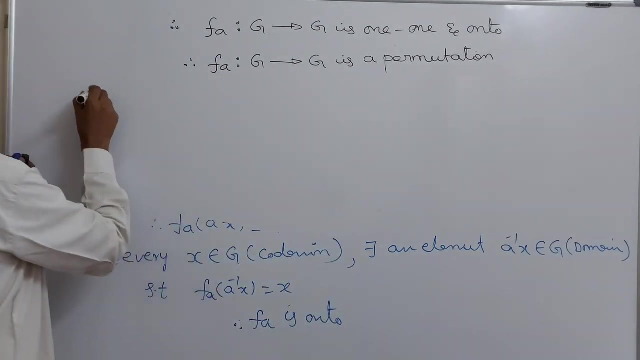 is nothing but a permutation. Therefore, fa maps G into G is a permutation, is a permutation on G, is a permutation defined on G. It is very clearly a permutation. 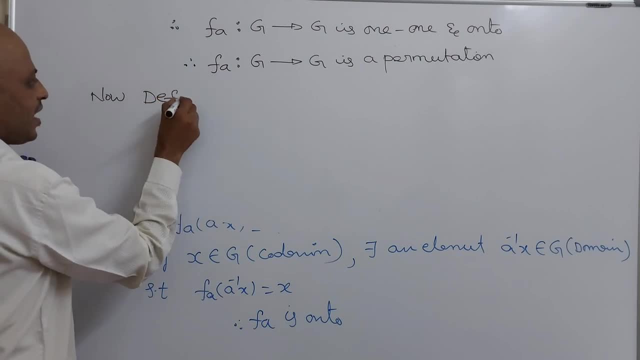 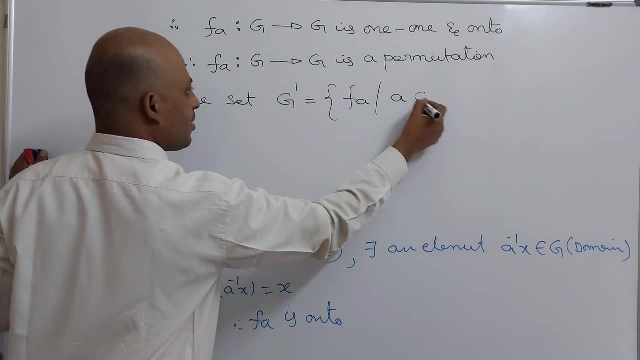 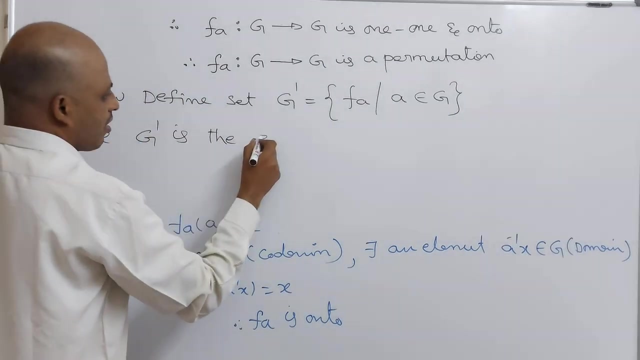 Now, define a set, now define a set G dash with all permutations fa such that a belongs to capital G. It means that is G dash is the set of all permutations, the set of all permutations. 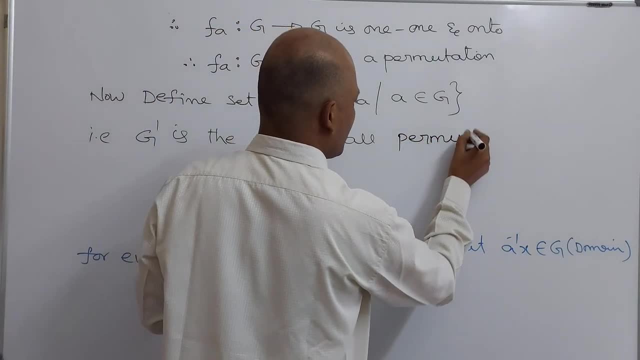 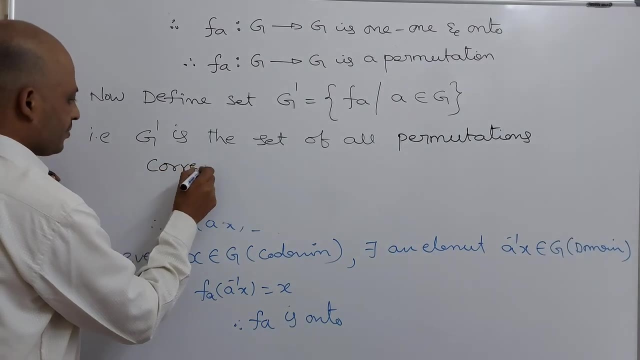 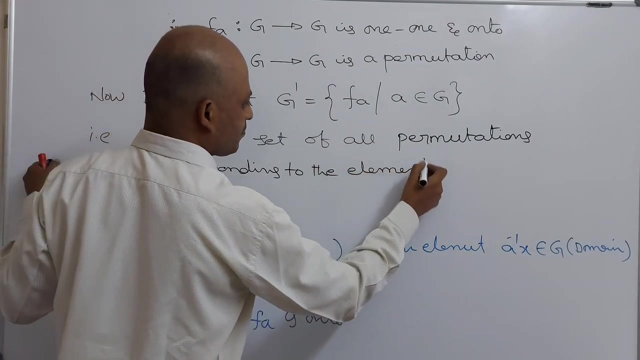 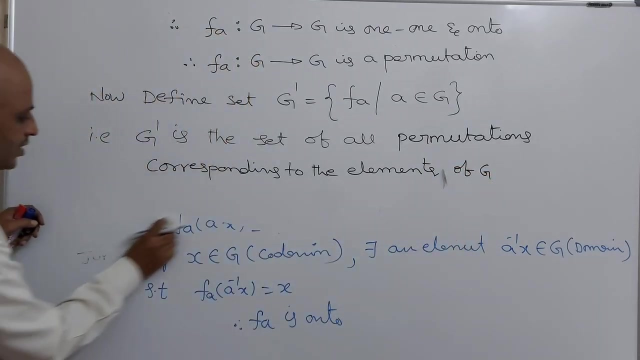 G dash is the set of all permutations. G dash is the set of all permutations corresponding to the elements of G corresponding to the elements of G. So, you have to understand like this. If G contains, if G contains three elements 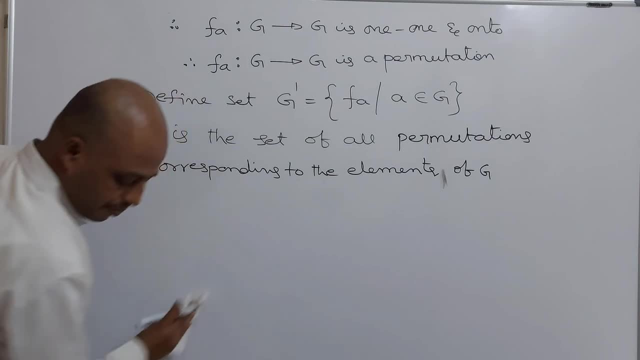 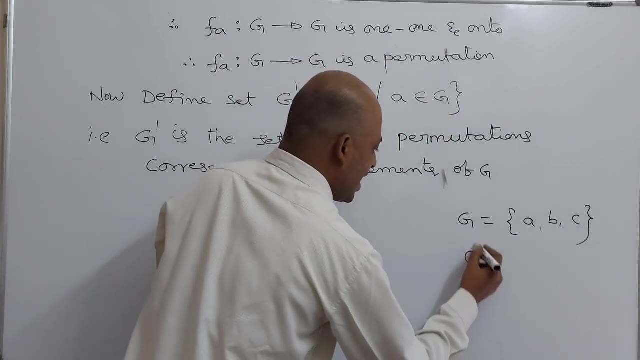 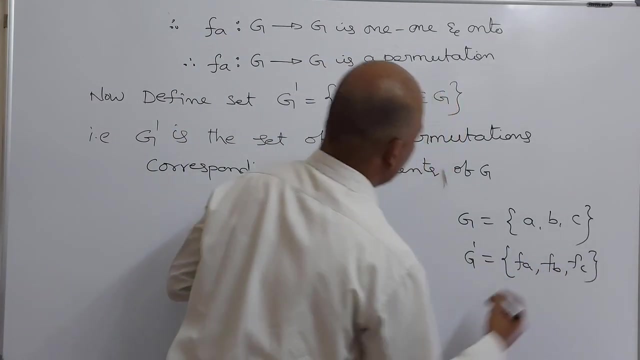 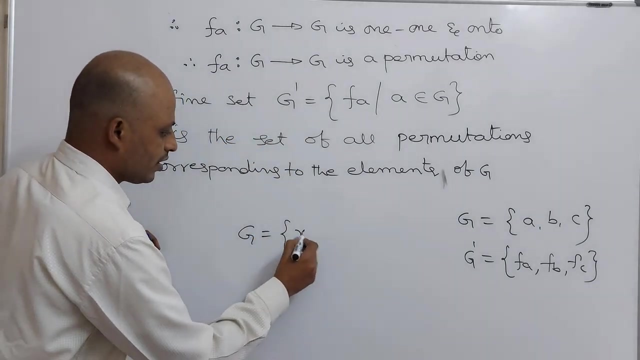 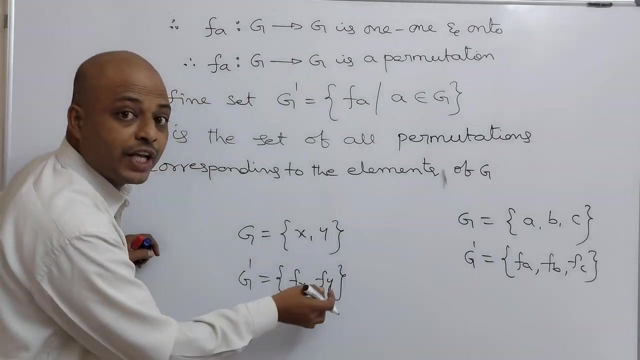 a b c, you have to understand like this. Suppose, suppose G contains three elements a comma b comma c, then G dash contains only three elements which are permutations fa, f b, f c. That is all. The set G dash defined like this. If G contains only two elements x y, then G dash contains again two elements only f x and f y which are permutations, which are permutations on G, which are permutations on G. .. 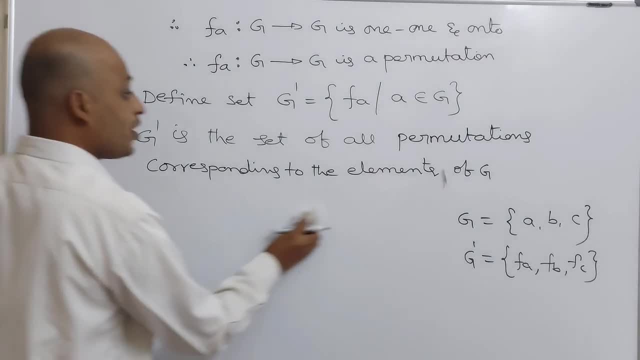 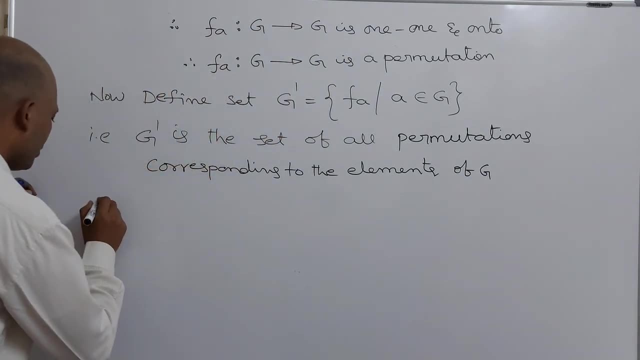 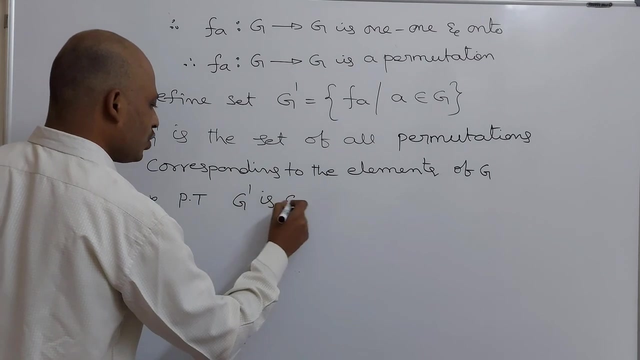 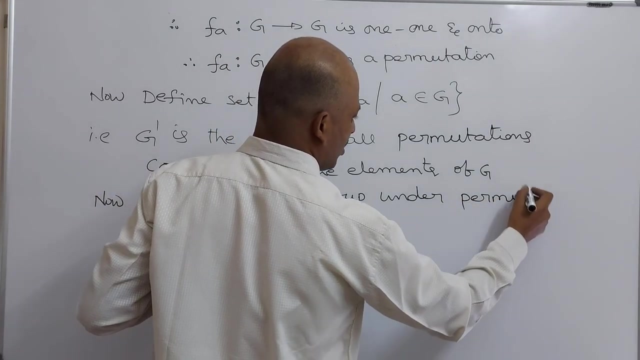 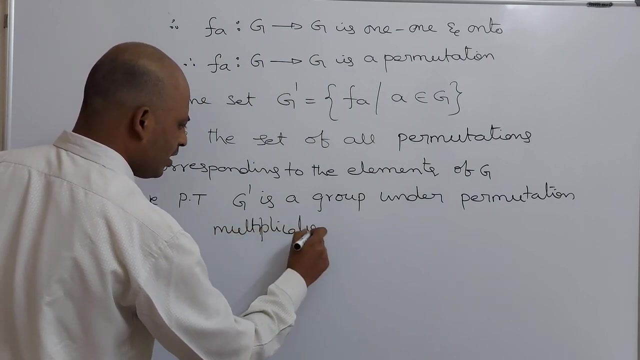 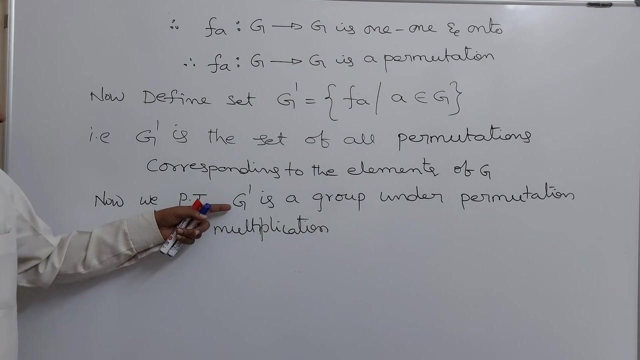 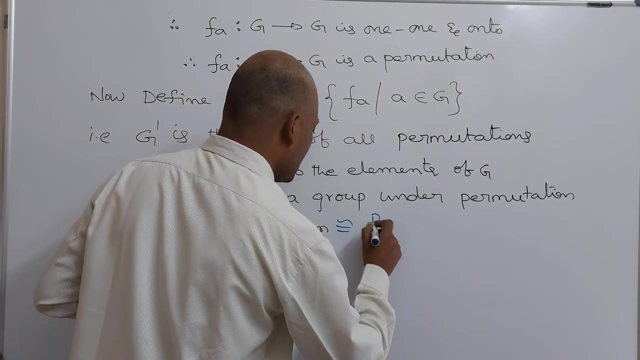 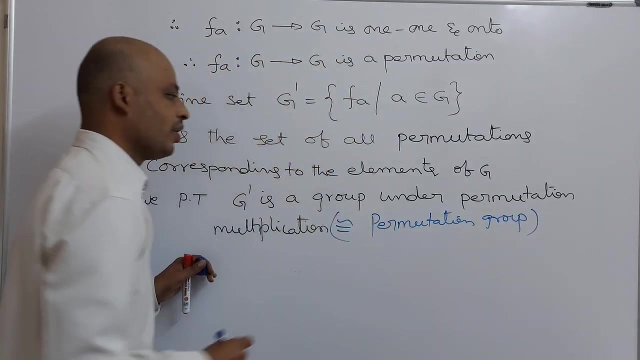 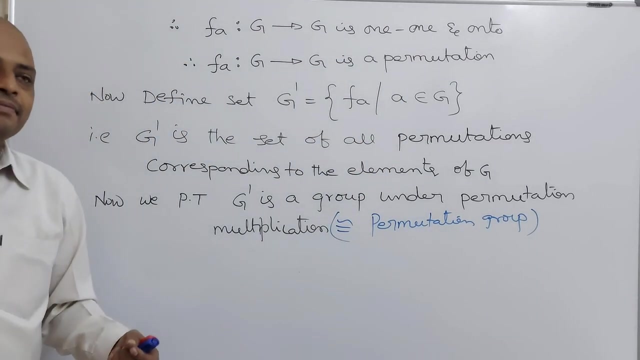 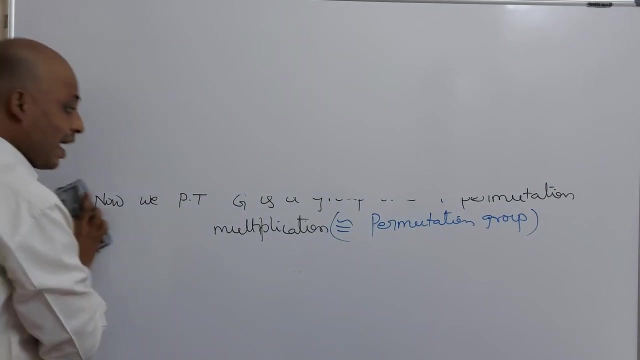 dash is the set of all permutations corresponding to the elements of G. We prove that. Now this is the first part of our theorem. So we define the set G dash. In the second part we prove that this set G dash. Now we prove that G dash is a group. G dash is a group under permutation multiplication. Under permutation multiplication. G dash is a group under permutation multiplication. In the second part we prove that this group G dash is. We prove that this set G dash is a group under permutation multiplication which is known as permutation group. Which is known as permutation group or symmetric group. Which is known as permutation group or symmetric group. Yes. We know that the group axioms closure, associative, identity, inverse and inverse axiom. That if you show that the four axioms holds in G dash then it is a group. Let us start with closure axiom. 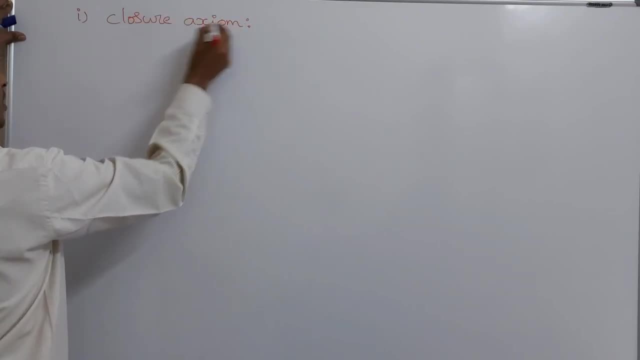 Closure axiom. To prove that closure axiom take two elements a ,b belongs to capital G. For a ,b belongs to capital G we have the element also a,b belongs to capital G. The 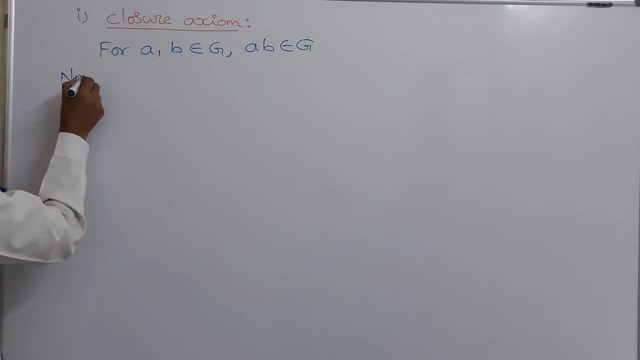 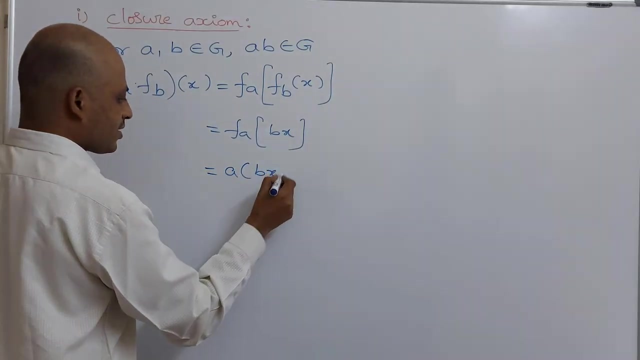 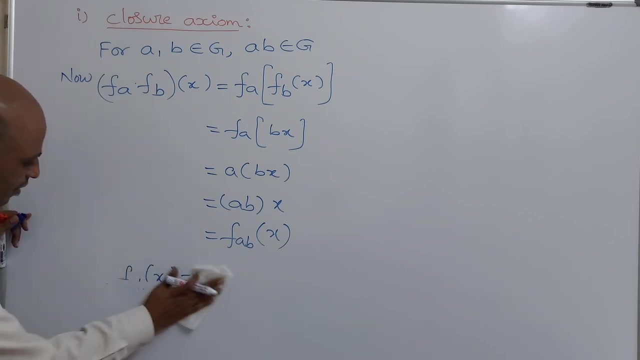 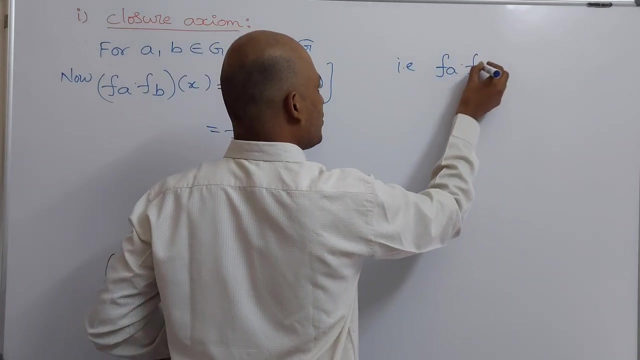 element also a,b belongs to capital G. Now calculate f a into f b. f a into f b of x is by the product of permutations it can be written as f a of f b of x f a of b x it is this is nothing but a into b x this is nothing but a b into x this is nothing but f a b of x therefore finally we prove that f a b of x is equals to sorry f a into f b of x left side we have f a into f b of x is equals to f a b of x that is that is f a into f b is equals to f a b 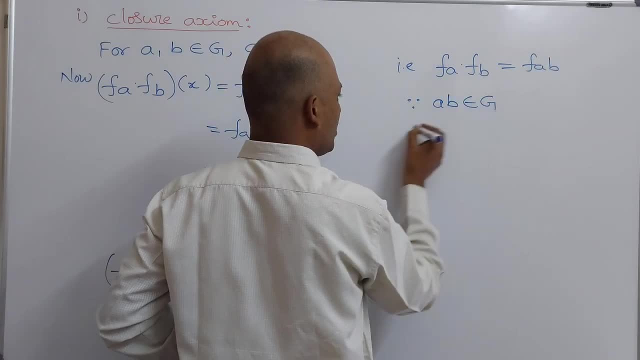 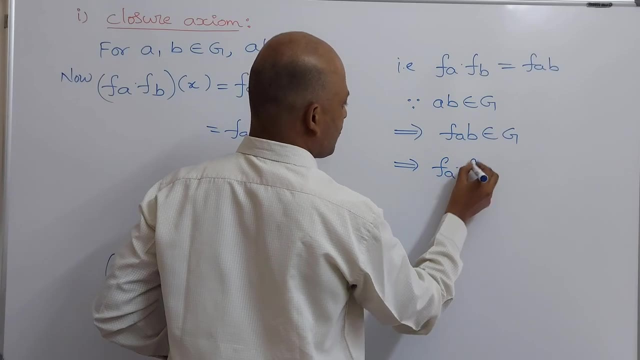 since a b belongs to capital g implies as f a b belongs to capital g implies as f a into f b belongs to capital g 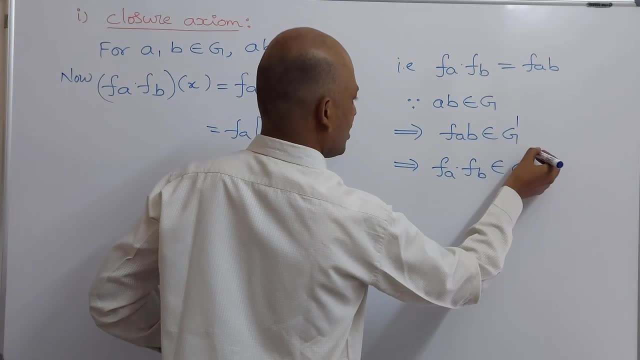 so this is g dash a b belongs to capital g f a b is a permutation remember that f a b is a 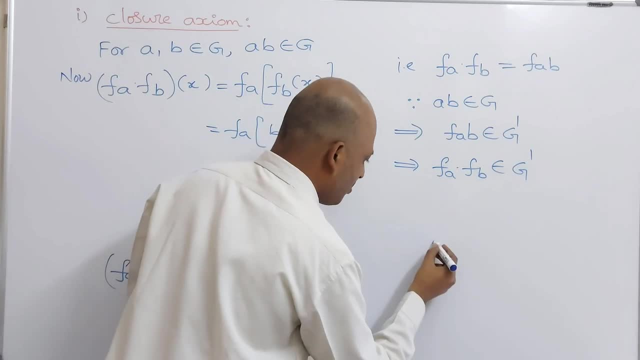 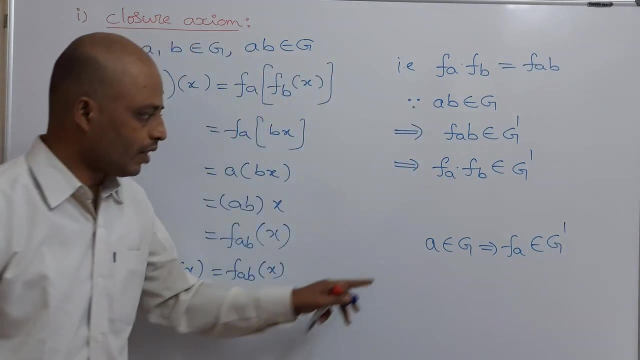 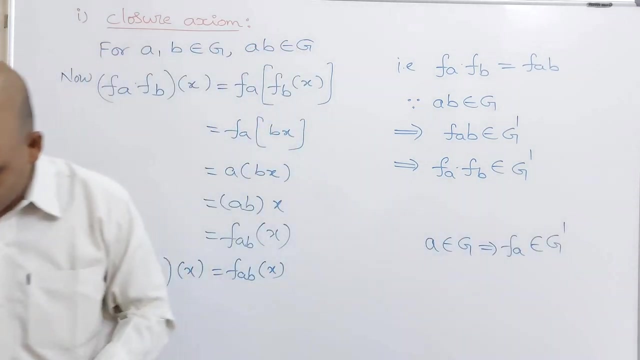 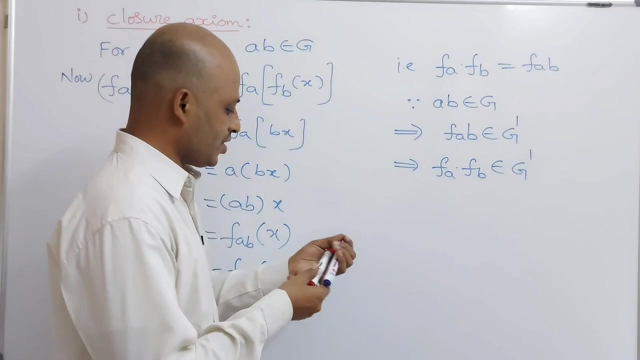 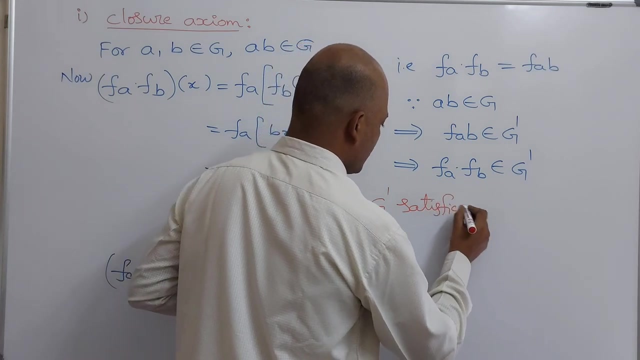 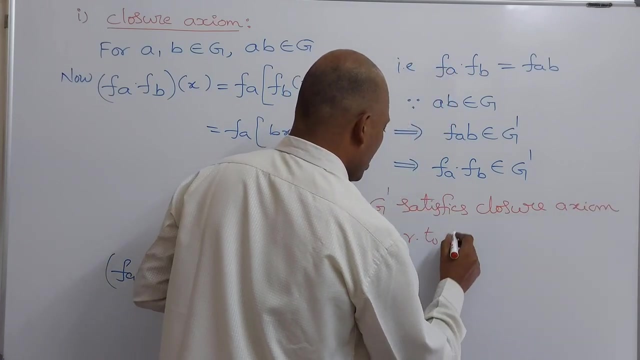 permutation a comma b are elements of g you remember the fact whenever a belongs to capital g f a is a permutation belongs to g dash whenever a belongs to capital g f a is a permutation that belongs to g dash that belongs to g dash please remember that so this condition shows us for the elements f a f b belongs to g dash therefore we said that g dash satisfies g dash satisfies closure axiom g dash satisfies closure axiom with respect to permutation multiplication with respect to permutation multiplication 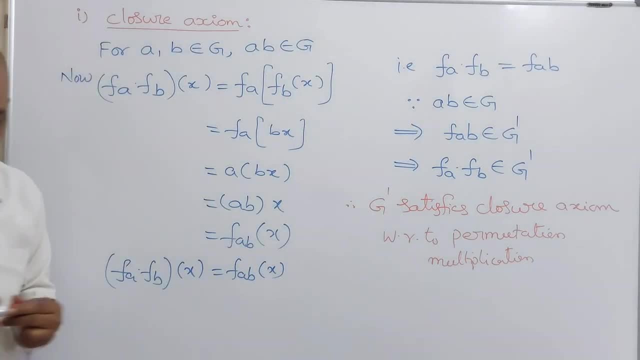 yes what is the second axiom in the group associative axiom 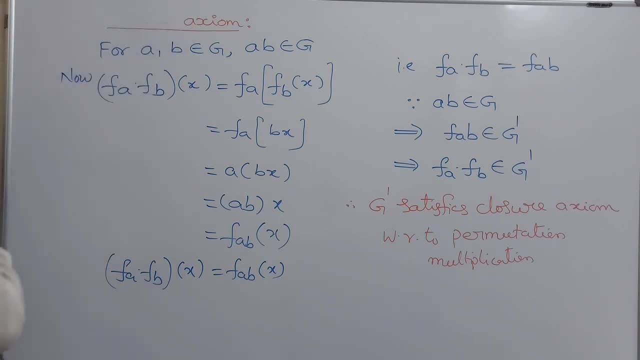 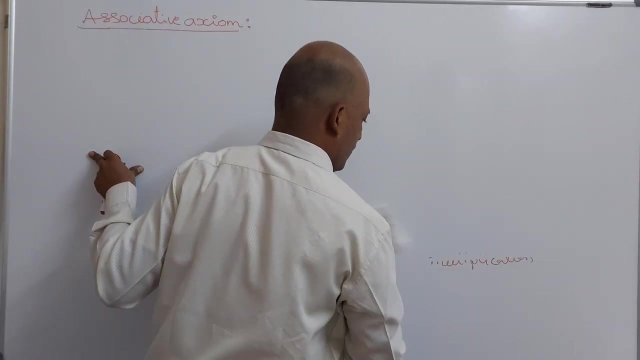 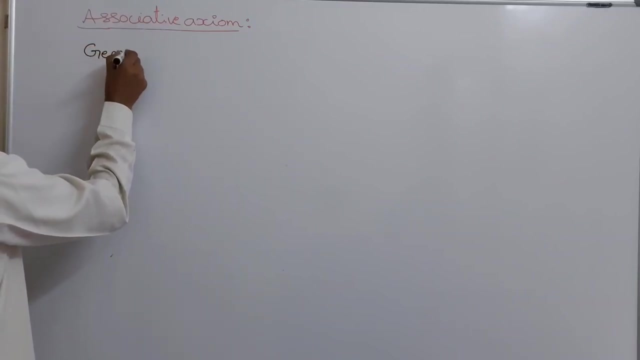 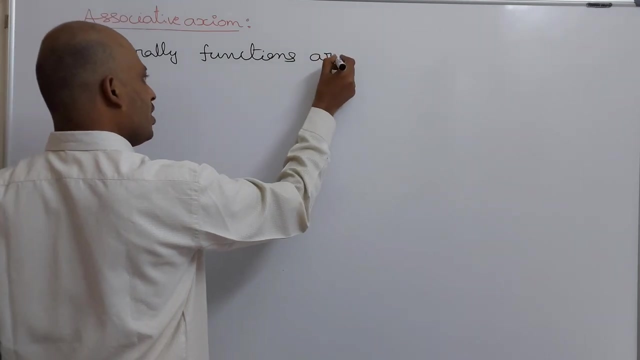 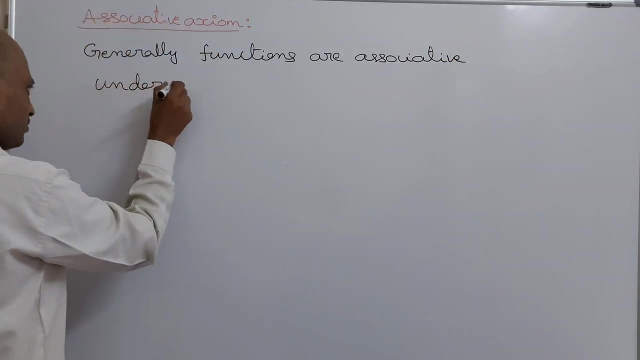 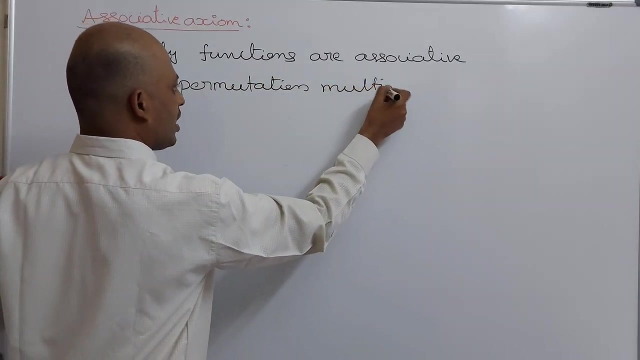 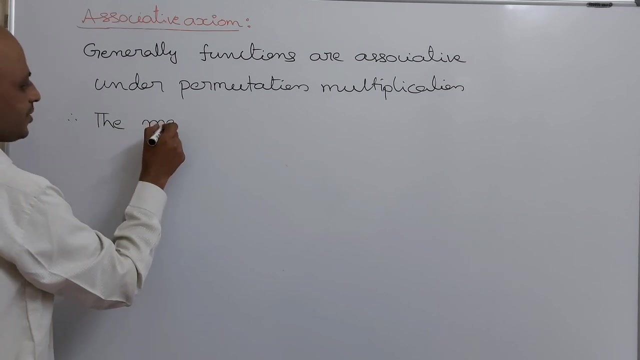 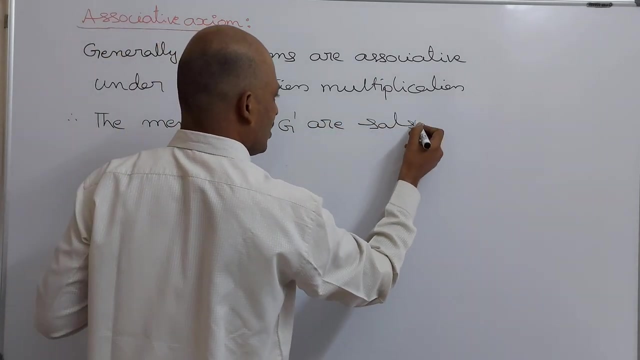 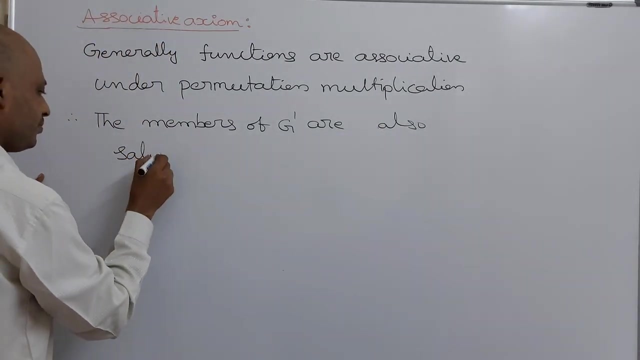 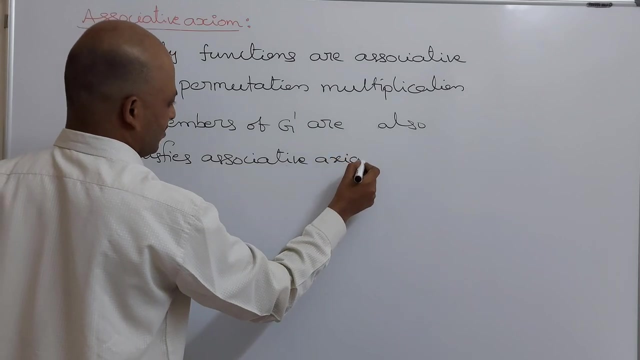 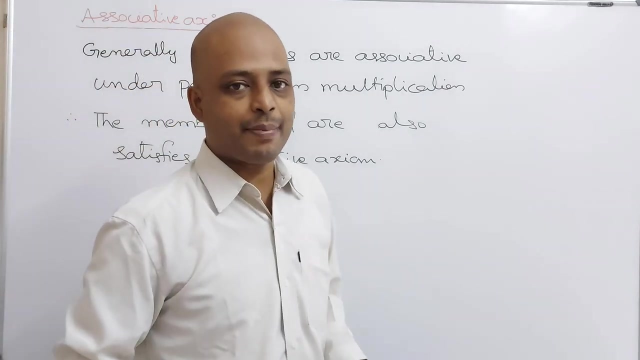 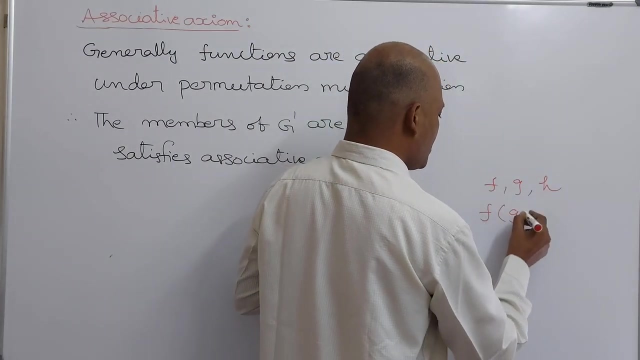 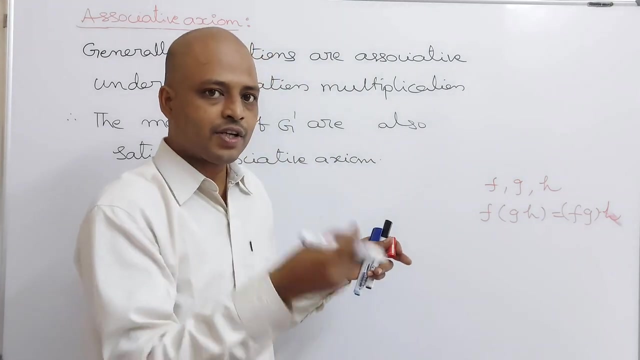 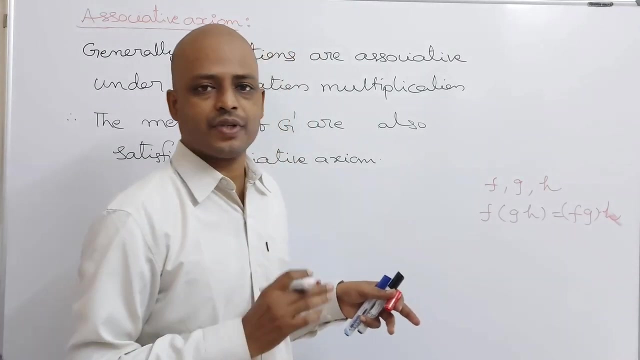 the group associative axiom associative axiom generally functions are associative so associative axiom is very very simple generally functions are associative generally functions are associative under permutation under permutation multiple under permutation multiplication therefore the members of g dash the members of g dash are also satisfies the members of g dash are also satisfies satisfies associative axiom associative axiom this is very simplest one we know that from intermediate level the product of the composition of mappings the product of mappings are associative suppose f g h are any three functions then f of g h is equals to f g of h f g of h this is general theory the product of functions or multiplication of functions or composition of functions is associative is associative 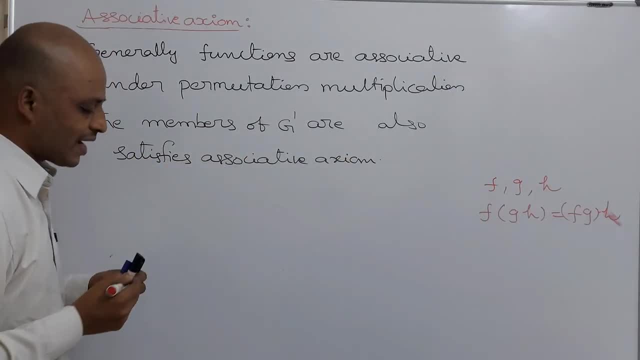 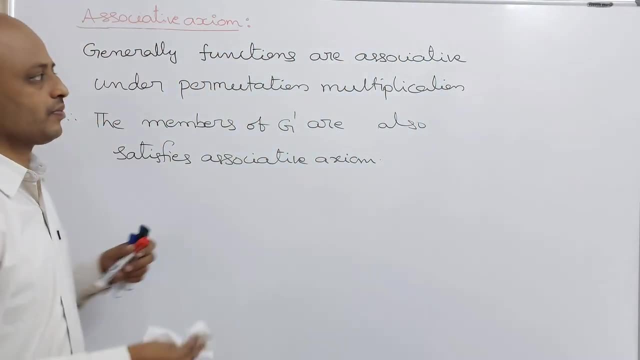 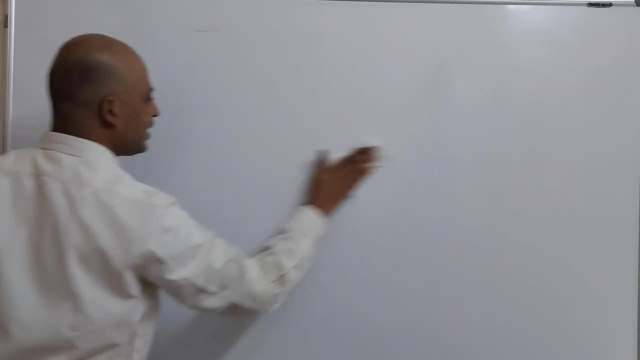 so the members of g dash are also satisfies associative axiom because members of g dash are nothing but functions permutation is nothing but a bijective function permutation is nothing but a bijective function what is the third axiom existence of identity 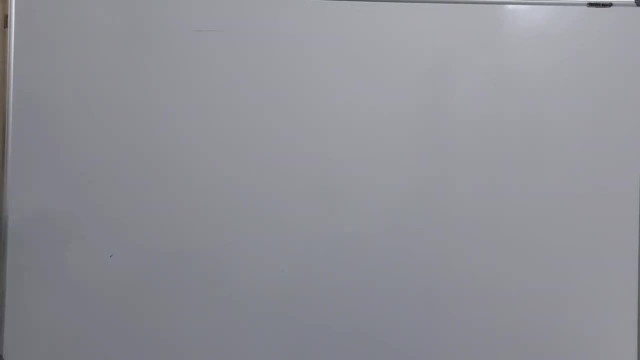 what is the third axiom existence of identity existence of 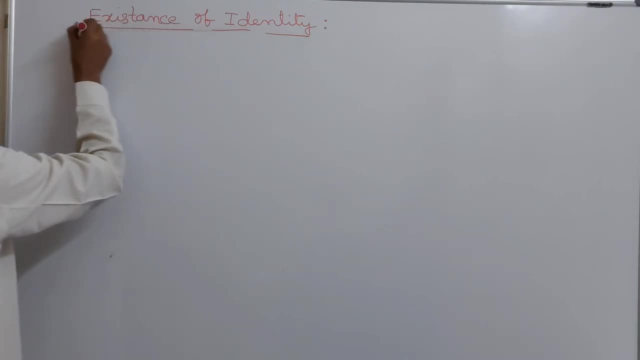 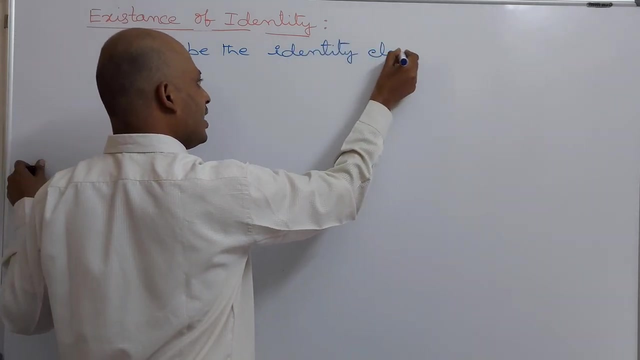 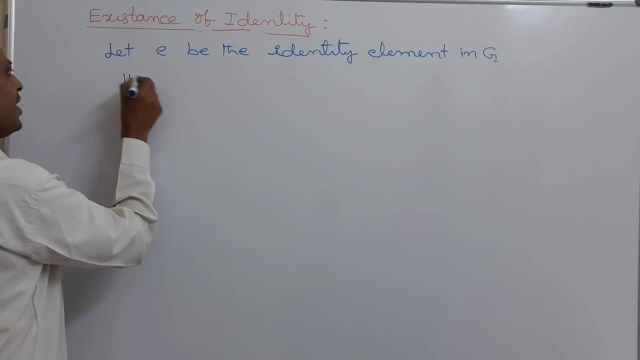 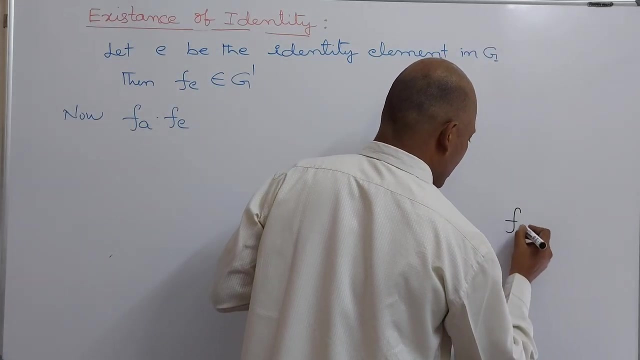 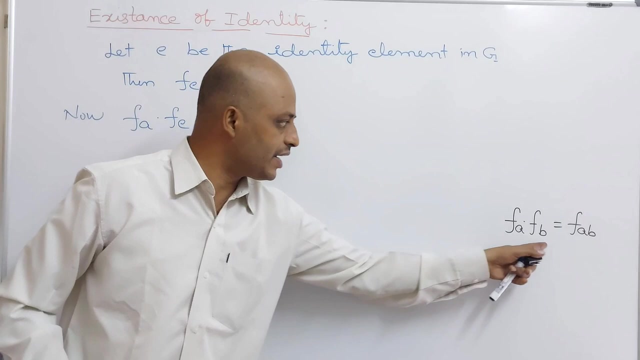 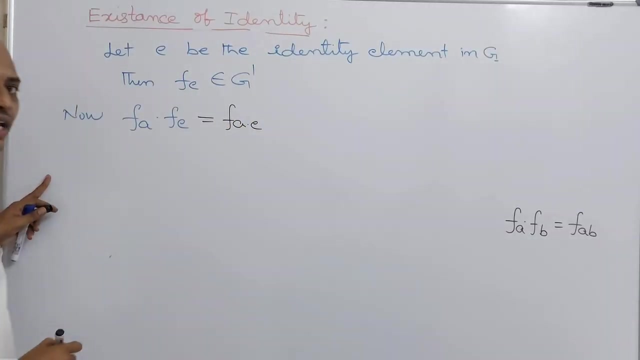 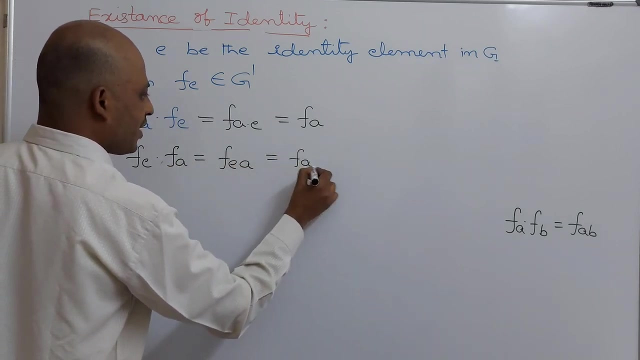 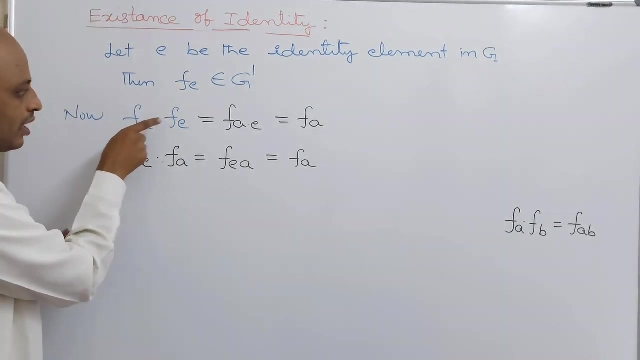 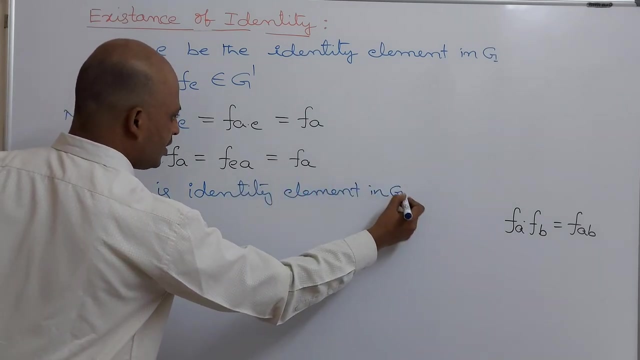 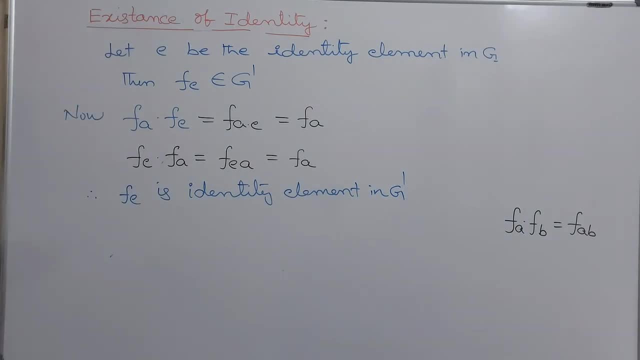 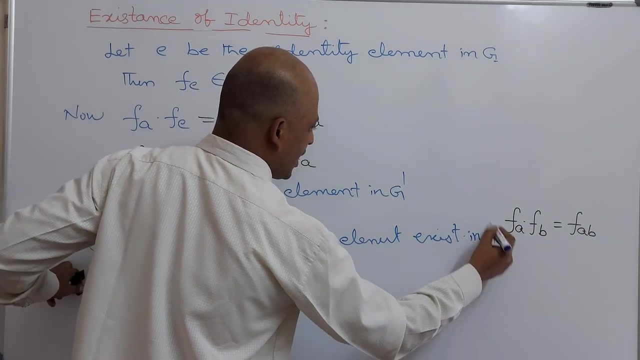 FE is identity element in G'. So, identity element exists in G'. Identity element exists in G'. Therefore, identity element exists in G'. 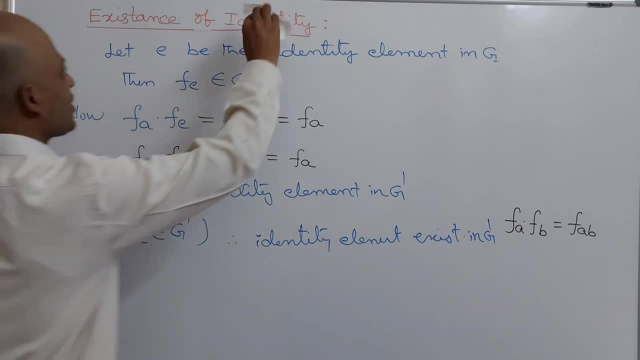 What is the fourth axiom in that group? Existence of inverse. 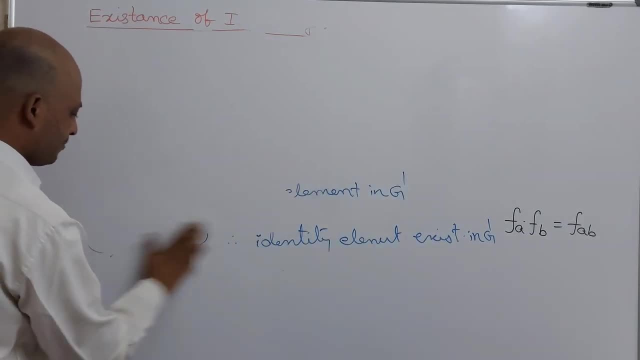 Existence of inverse. Let us solve that one. Existence of inverse. 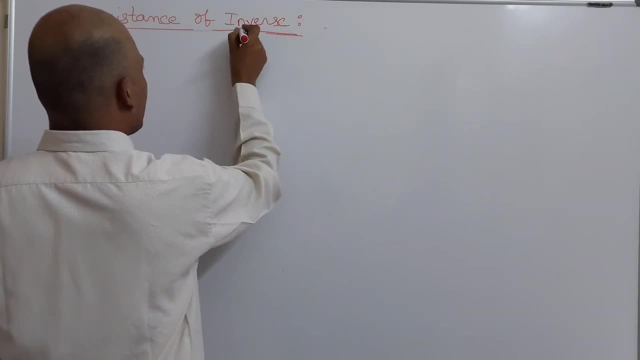 Existence of inverse axiom or existence of inverse. 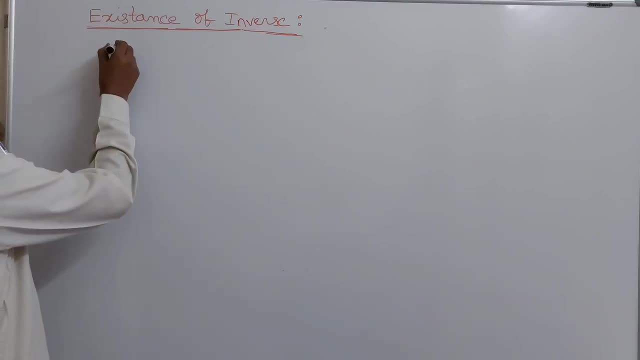 Let us take an element A belongs to capital G. Or since already we know that A belongs to capital G, apply the inverse axiom A inverse belongs to capital G. 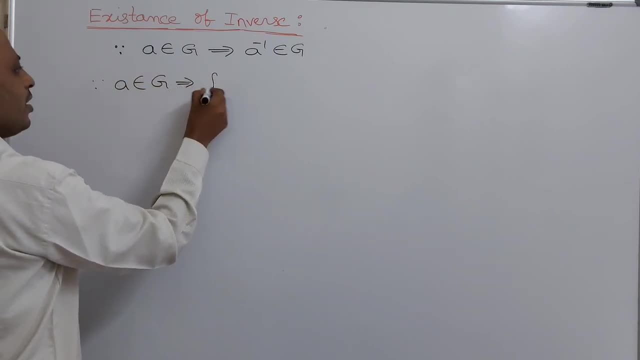 Since A belongs to capital G implies F A belongs to G'. A inverse belongs to capital G implies F A power minus 1 also belongs to G'. 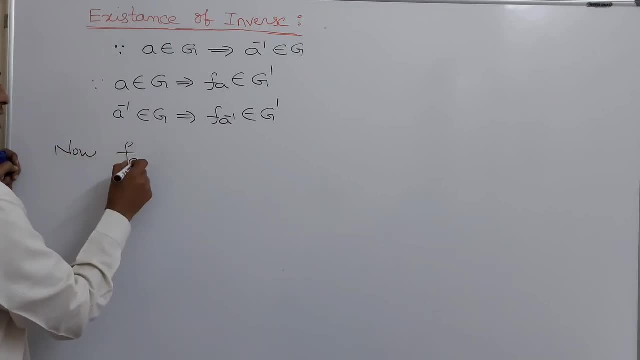 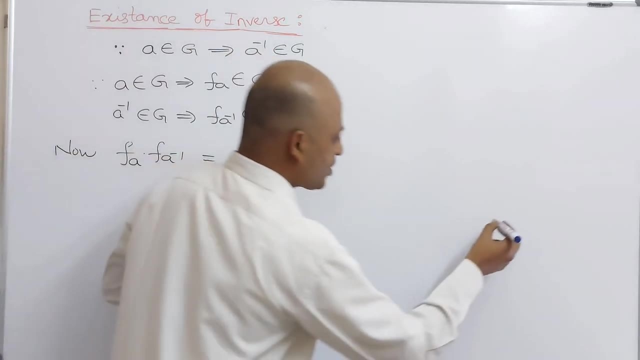 Now, calculate F A into F A inverse. F A into F A inverse. This is very trivial again by using this property. 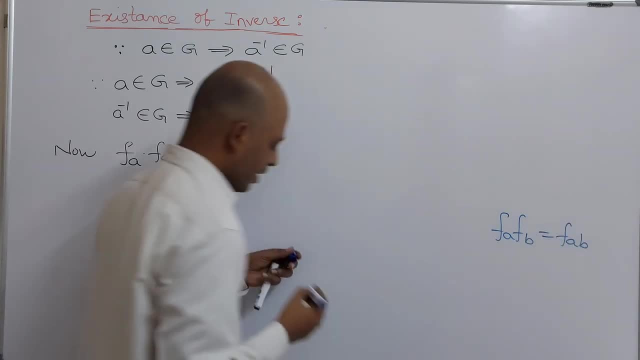 F A into F B is equals to F A B. F A into F B is equals to F A B. 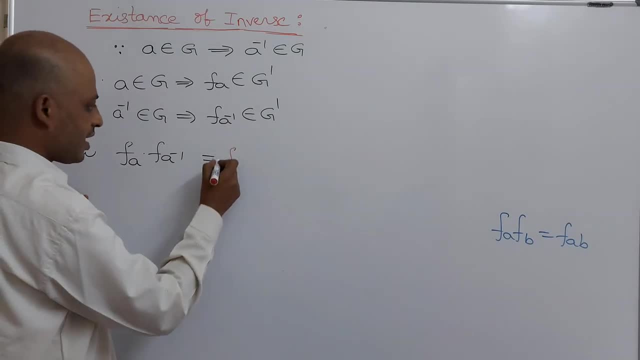 By applying this property, here F A into F A inverse can be written as F A A inverse. This is nothing but F E the identity element. F E the identity. 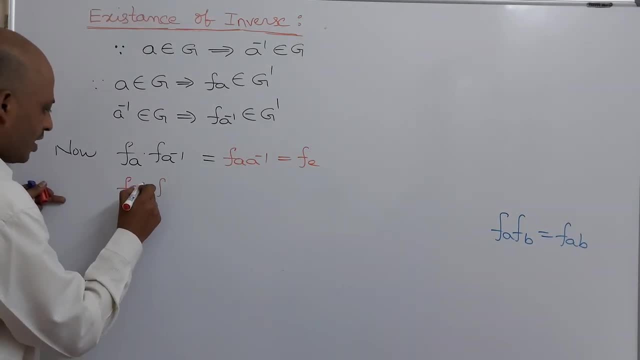 Similarly, you can prove that F A inverse into F A is equals to F A inverse A is equals to F E. So, by using these two equations, we conclude that 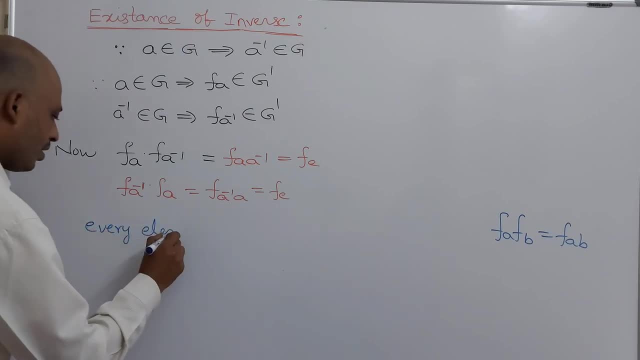 every element, every element F A belongs to G' has inverse F A power minus 1. 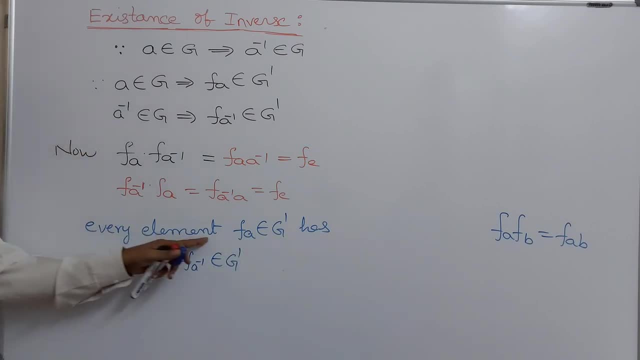 Every element F A belongs to G' has inverse F A inverse F A power minus 1. That also lies in the same set G'. 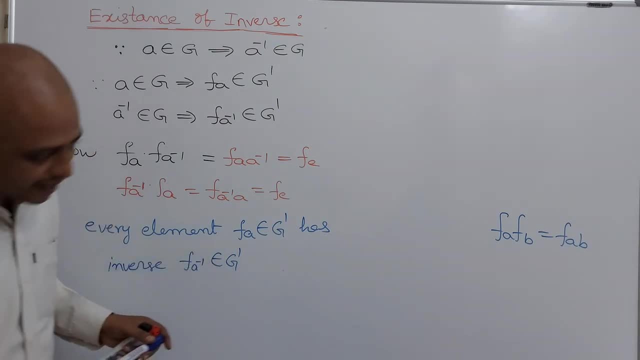 So, up to this one, we prove all the four axioms. We prove all the four axioms. Closure, associative, identity and inverse. 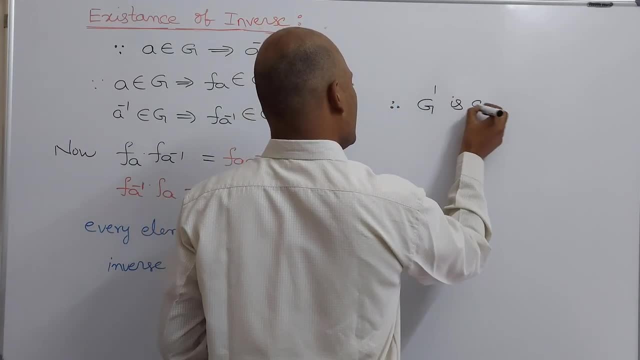 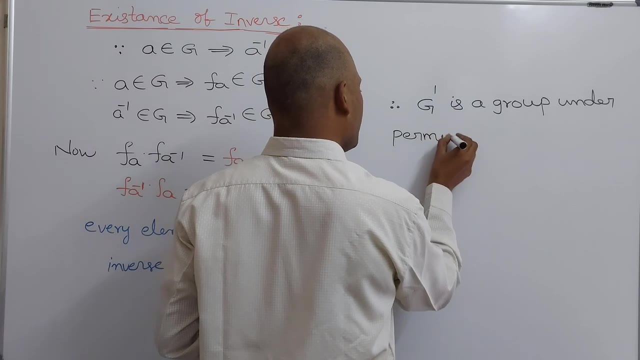 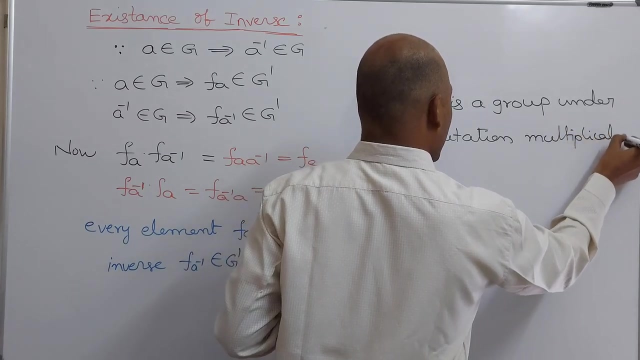 Therefore, we conclude that G' is a group. G' is a group. Under permutation multiplication, G' is a group under permutation multiplication, which is known as permutation group. 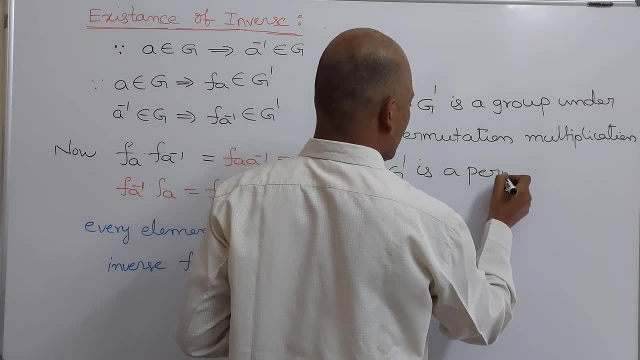 That is, G' is a permutation group. G' is a permutation group. 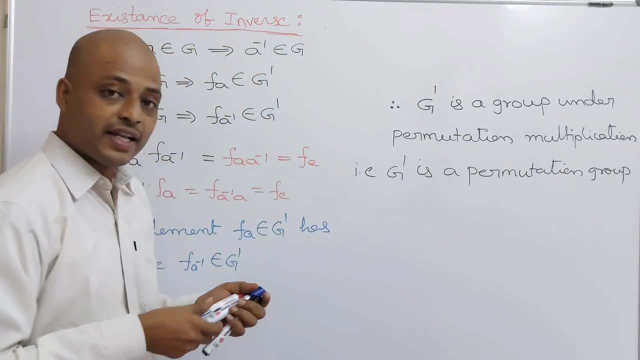 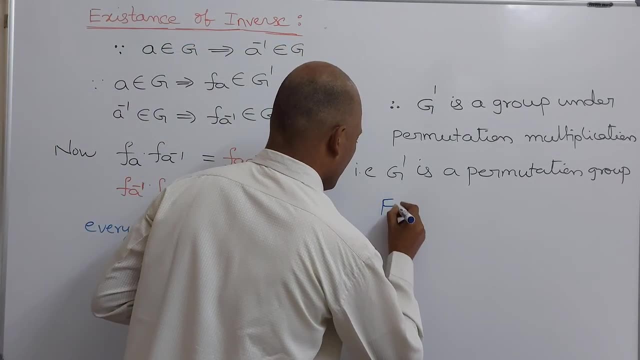 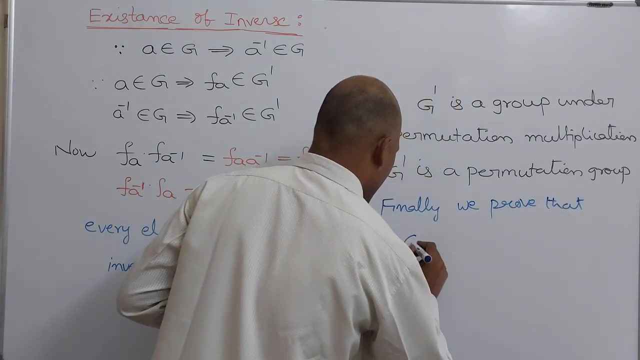 Finally, we prove that G' is isomorphic to C. Finally, we prove that G' is isomorphic to G. 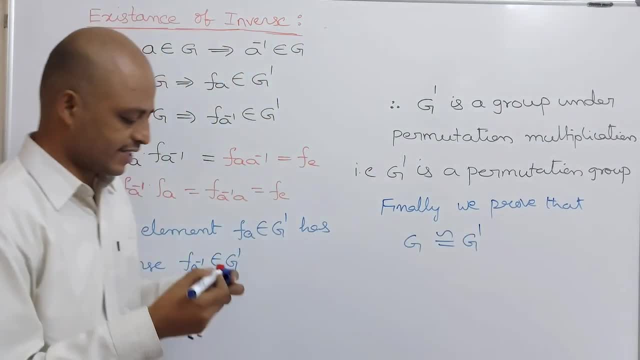 You can define G' is isomorphic to G. Both are same. G is a finite group. G is a finite group. G' is a permutation group. 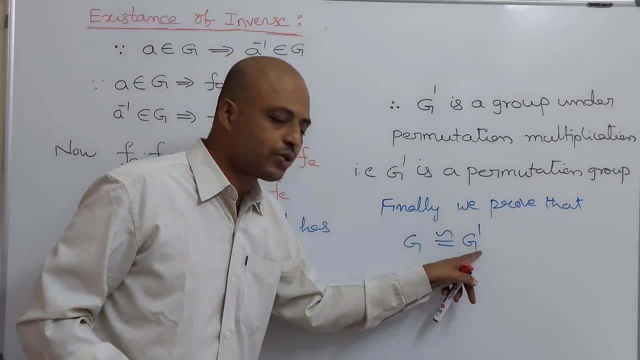 It means every finite group G is isomorphic to a permutation group G'. I have written it. I have written it. I have written it again. 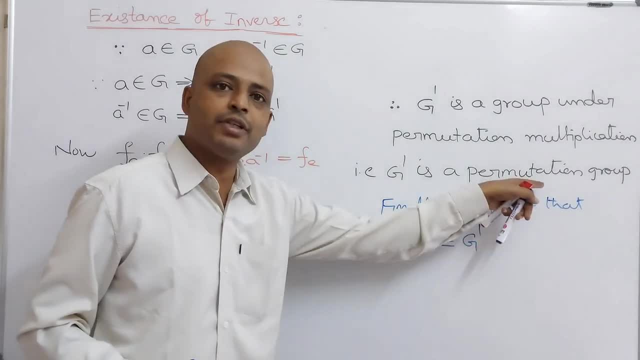 G is a finite group. G' is a permutation group. 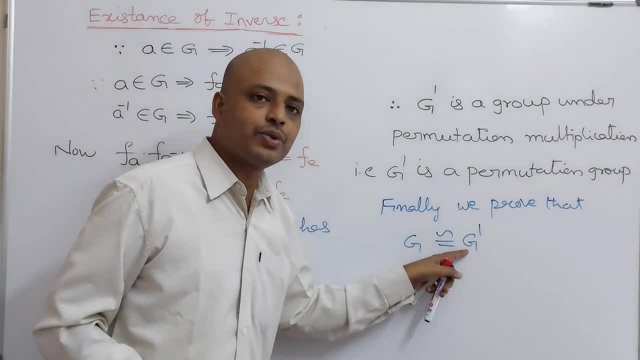 It means every finite group G is isomorphic to a permutation group G'. 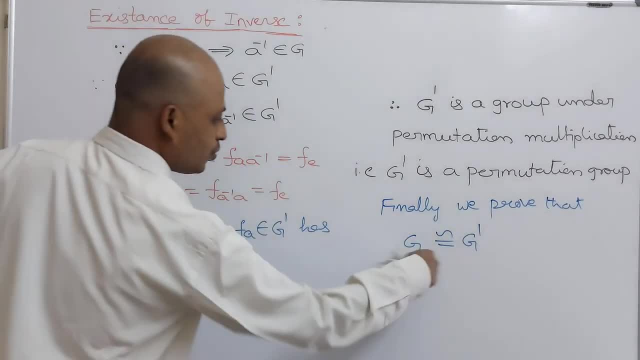 To prove this, define a mapping. To prove this, G is isomorphic to G'. 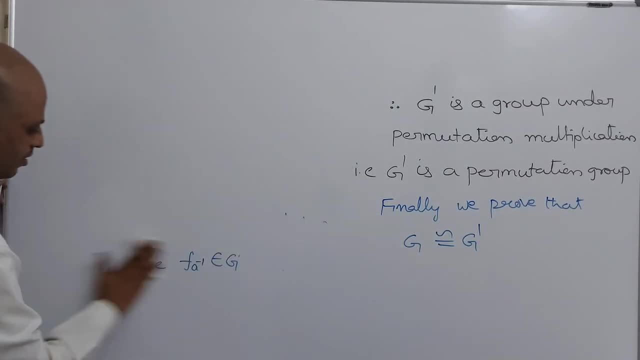 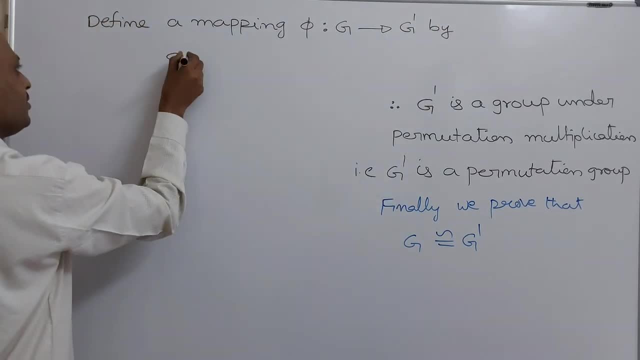 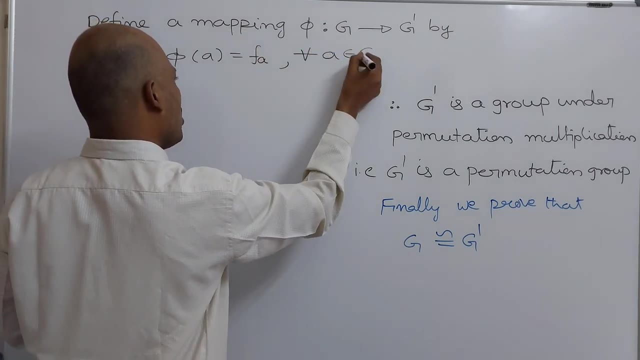 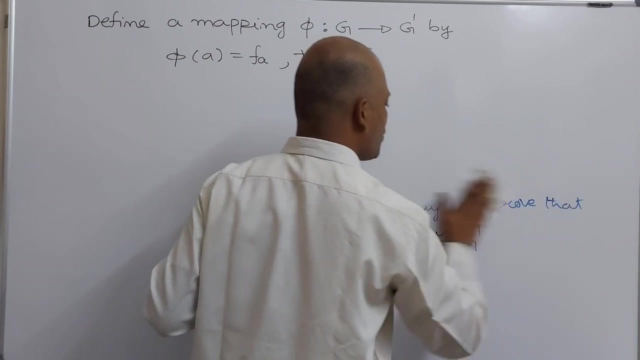 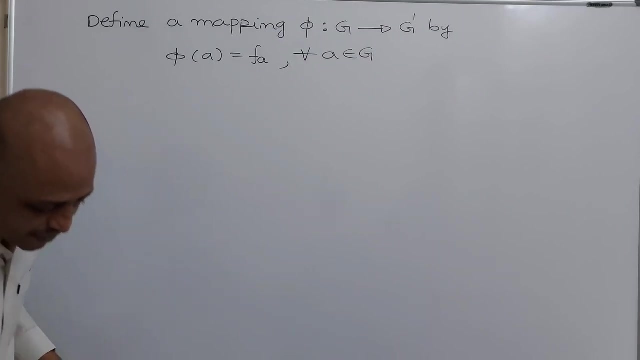 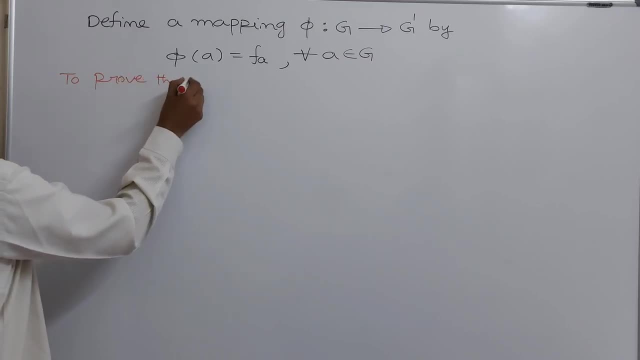 To prove that pi is 1-1. To prove that pi is 1-1. Simple proof. 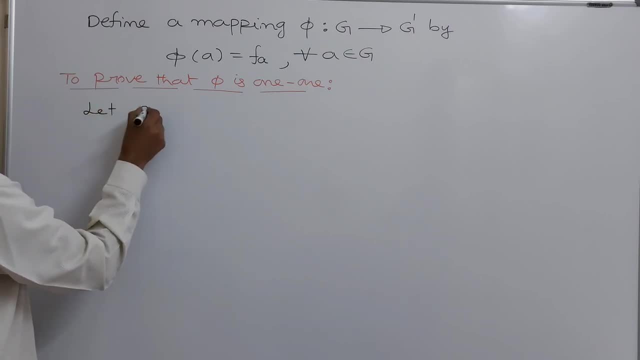 Let us take a, b belongs to capital G. a, b belongs to capital G. 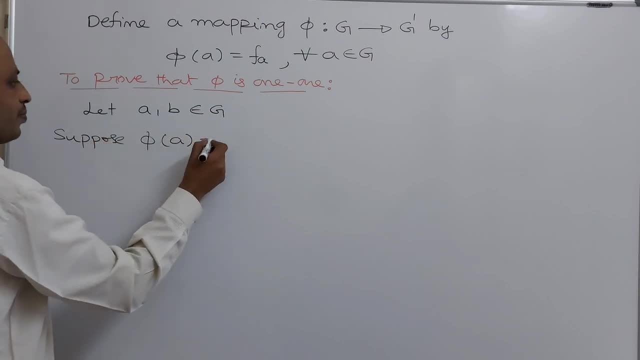 Suppose pi of a is equal to pi of b. 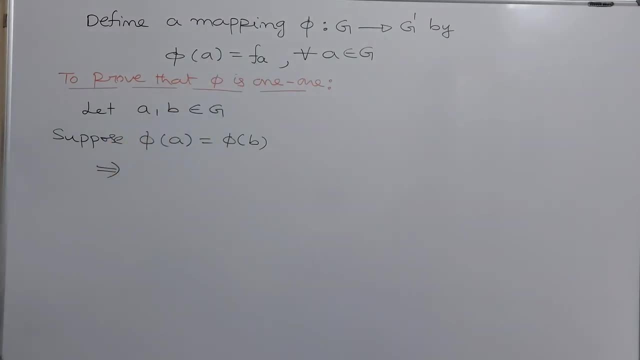 Which implies by definition pi of a is equal to f of a. Which implies by definition pi of a is equal to f of a. 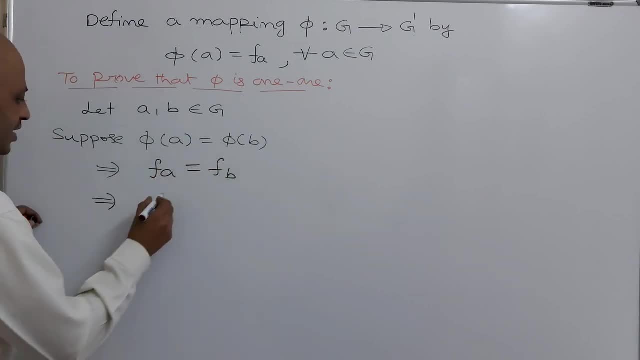 F A is equals to F B. F A is equals to F B means F A of x is equals to F B of x, which is nothing but A x is equals to B x, which is nothing but A is equals to B by right cancellation law, by right cancellation law. Therefore, we conclude that pi of A is equals to pi of B implies as A is equals to B. This shows as pi is 1, 1. This shows as pi is 1, 1. After 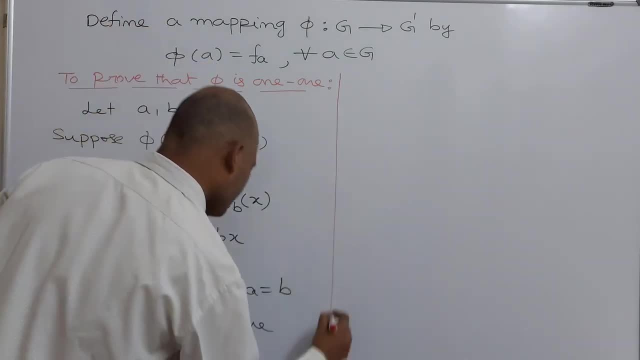 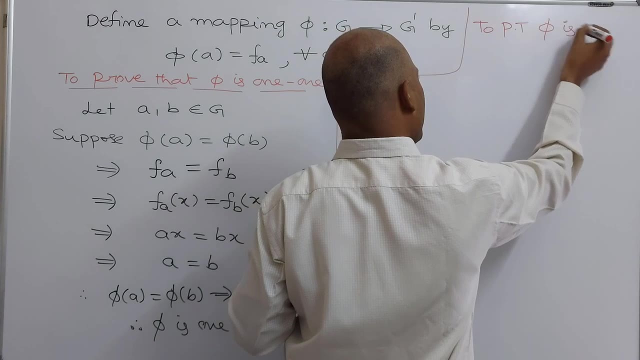 pi is 1, 1, we prove that pi is onto. We prove that pi is onto. To prove that pi is onto. 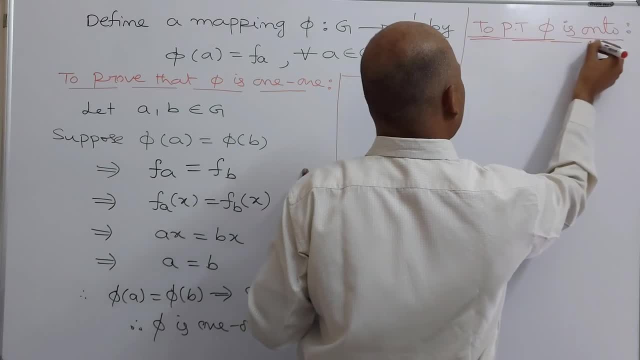 Very, very simple. What is the definition of onto? Every element of the codomine has at least one preimage in the codomine. So, every element of the codomine has at least 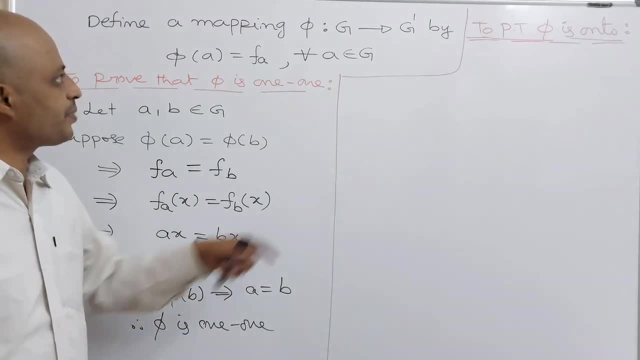 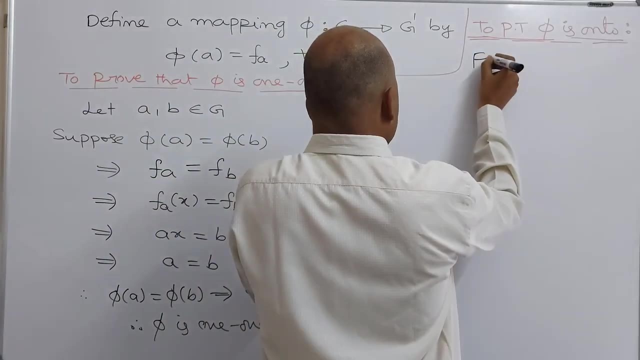 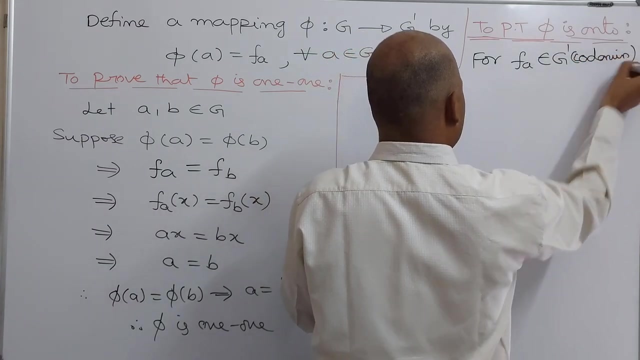 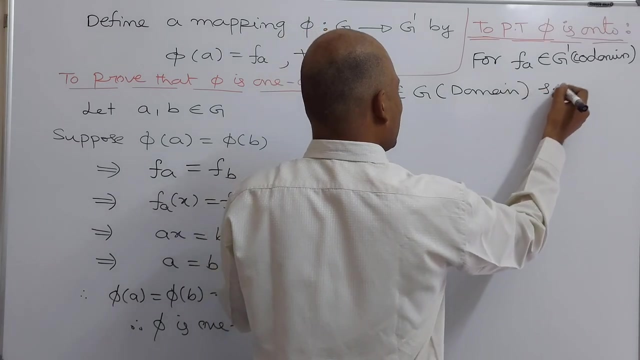 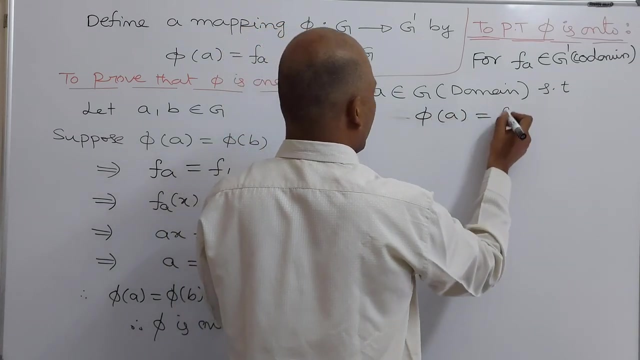 one preimage in the codomine. What is codomine? G dash. What is codomine? G dash. For F A belongs to G dash codomine, for F A belongs to G dash codomine, there exists an element A belongs to G domain such that F A such that pi of A is equals to A x is equals to pi of F A. Pi of A is equals to F A. It means every element belongs to the co-domain. Has at least 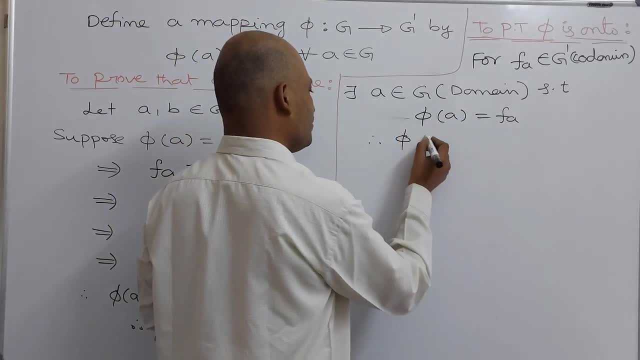 one pre-image in the domain. Therefore pi is onto. Therefore pi is onto. Right. Next 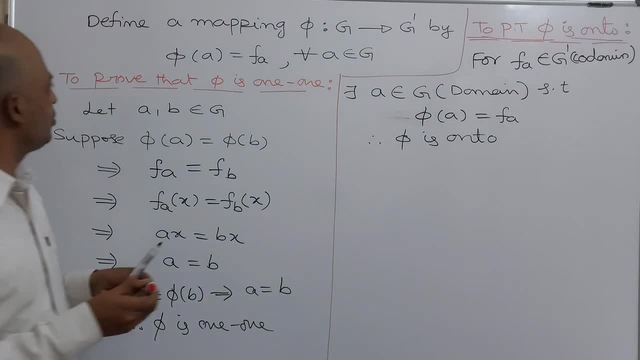 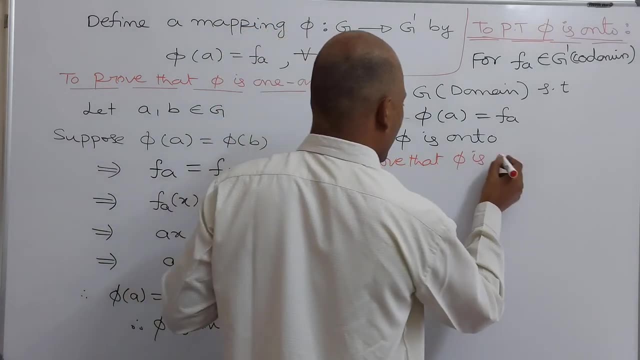 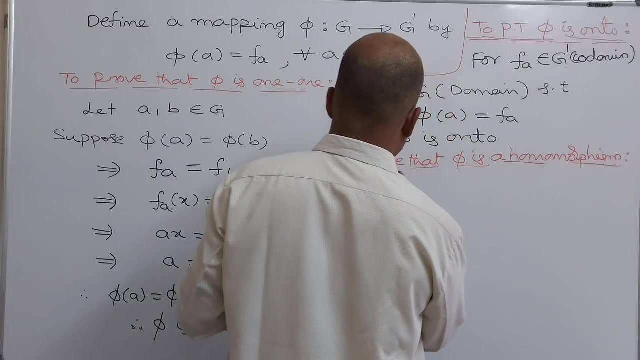 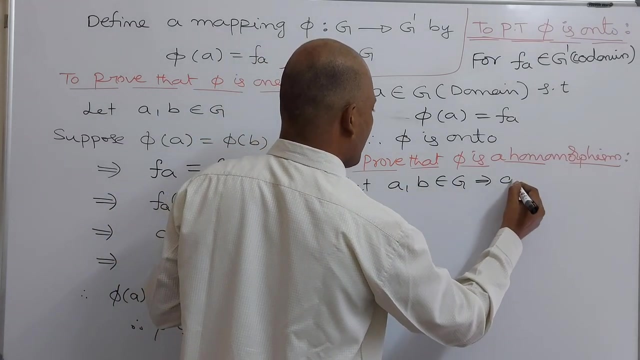 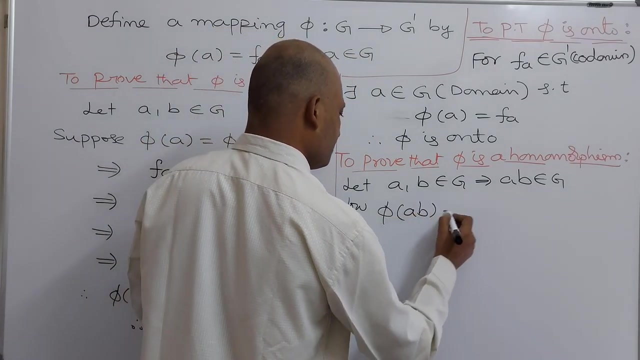 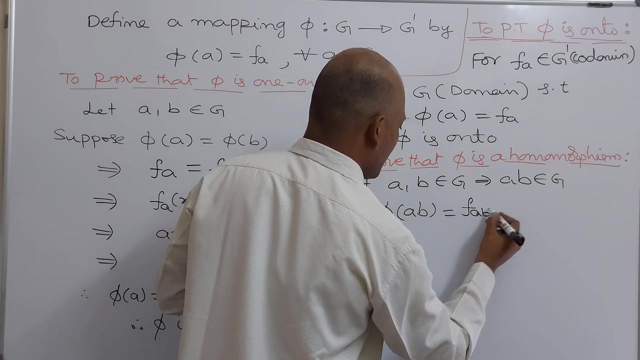 we prove that pi is a homomorphism. To prove that pi is a homomorphism. To prove that pi is a homomorphism again take two elements. Let us take any two elements A comma B belongs to capital G. By closure axiom A B also belongs to capital G. Now consider pi of A B. Pi of A B. By definition of pi, pi of A is equals to F A. So you can write F A B. Already we proved that pi is a homomorphism. To prove that pi is a homomorphism again take two elements. 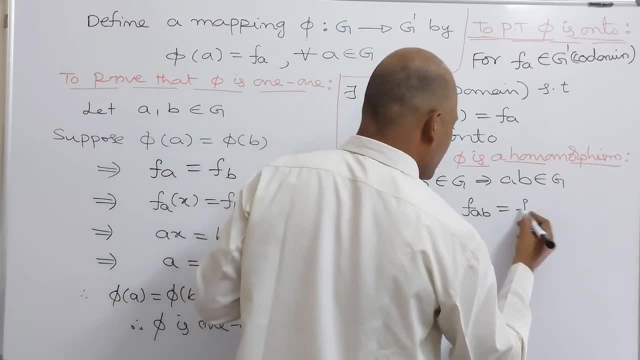 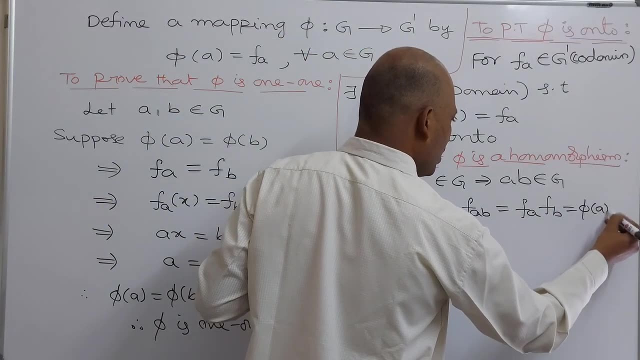 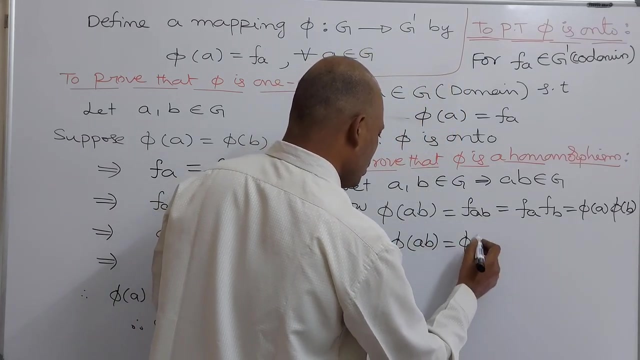 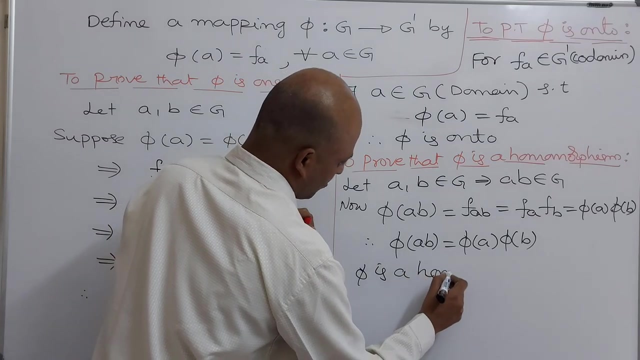 So we prove that in the closure axiom F A B can be written as F A into F B. F A into F B. This F A is nothing but pi of A. This F B is nothing but pi of B. Therefore we prove that pi of A B is equals to pi of A into pi of B. Therefore pi is a homomorphism. Pi is 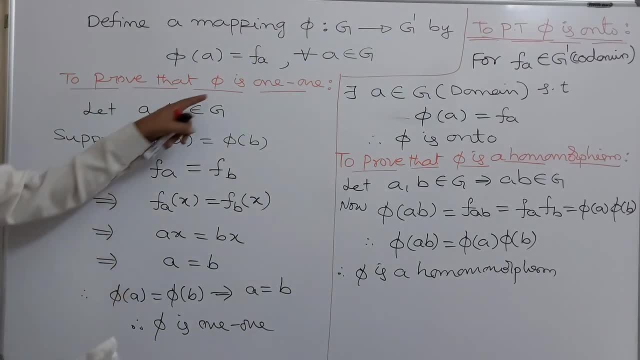 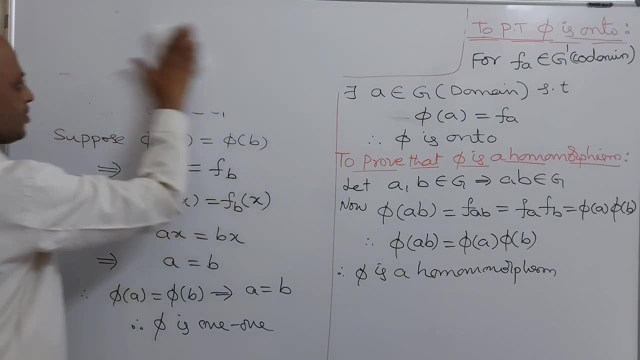 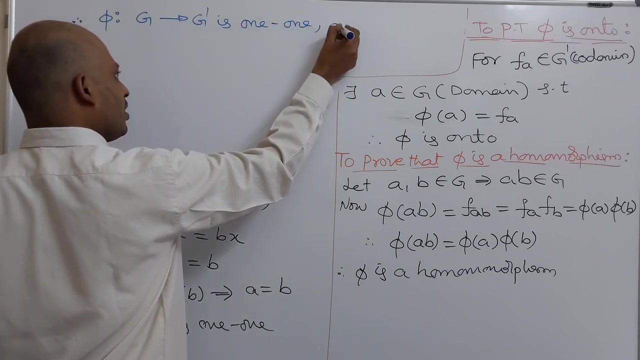 equals to pi of A 2. So we observe that. So now we show that it is a one-one function. It is onto function. It is homomorphism also. It is homomorphism also. Therefore pi max g into g dash is one-one comma onto and homomorphism and homomorphism also. So now we prove that pi x into g dash is one-one comma on-two and homomorphism and homomorphism also. This is J equal to p x G合 gmax, c equal to q over 1. 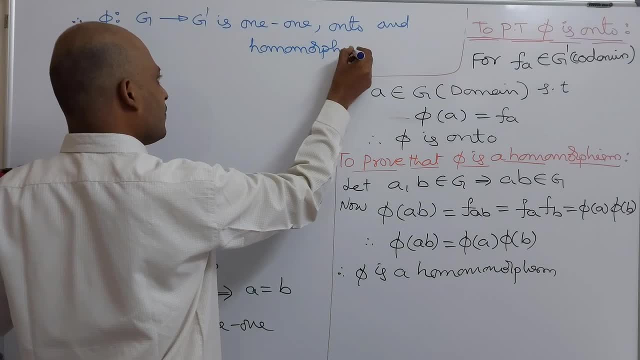 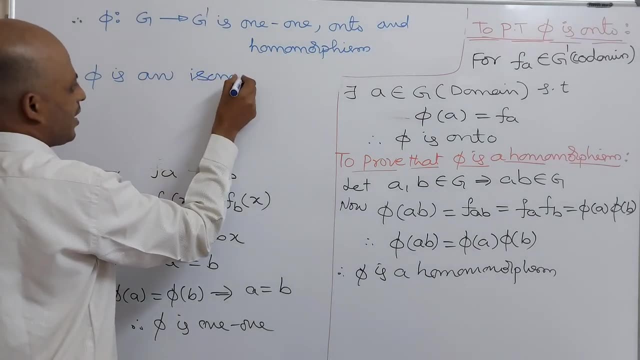 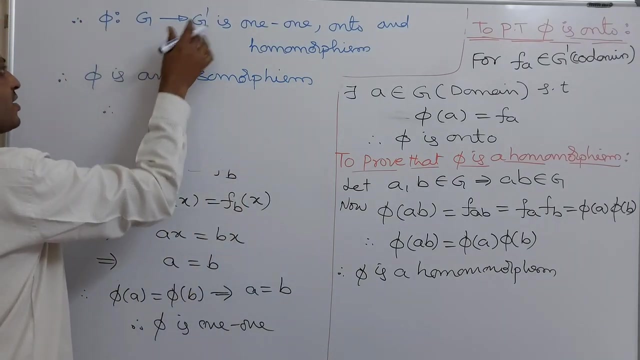 homomorphism. Therefore, pi is an isomorphism. Pi is an isomorphism. We know that if pi is an isomorphism, then G is isomorphic to G dash. Then G is isomorphic to G dash. This completes the 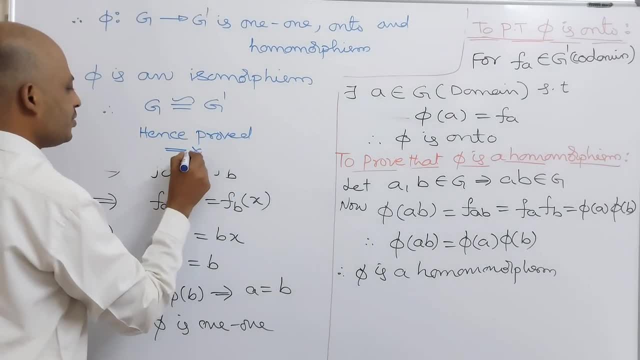 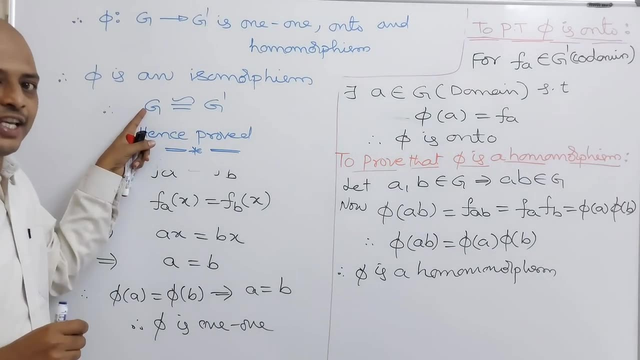 proof. Hence true. We discussed the detailed proof of the Cayley's theorem. You observe that in the left side, G is a finite group. In the left side, G is a finite group. In the right side, 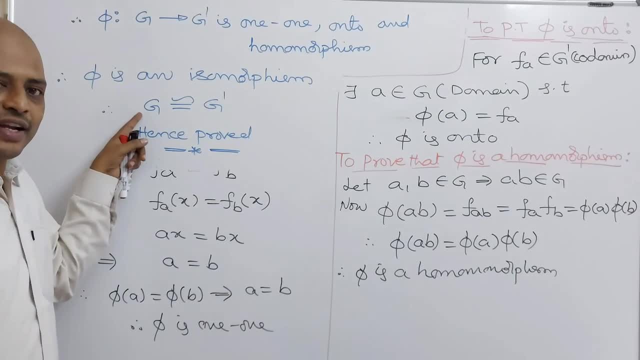 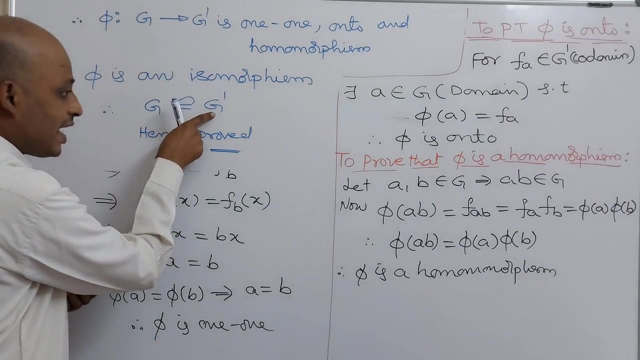 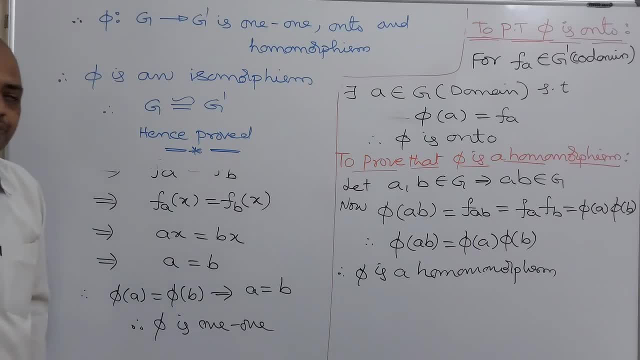